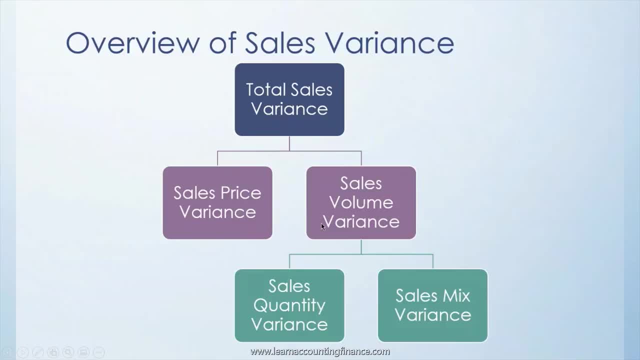 on the other hand, reflects the change in quantities. So you have a budgeted quantity but actually your sales is different, So you have a different actual quantity. This reflects sales volume variance. Now, within sales volume variance, there are two factors. 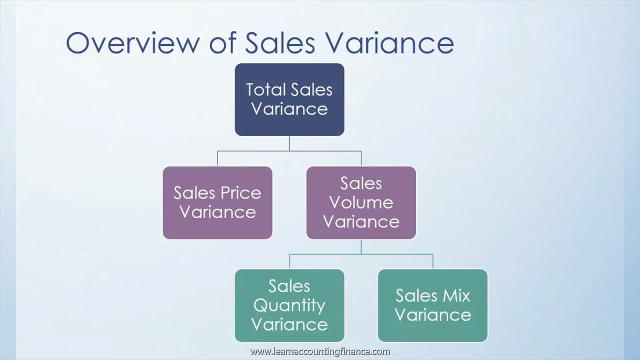 What you will see in the example that we'll see, in the example that we'll see in the example that we'll follow, is that we have sales where we have multiple products. We do not only sell one product, but we sell multiple products, And in that case, what becomes an important factor? 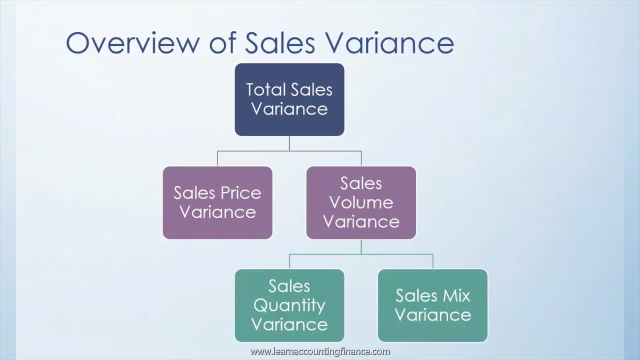 is how much of each product do we sell compared to our benchmark or our reference point, which in this case, is budget. So remember, we are comparing actual versus budget. How many actual sales of each product did we do versus what was in the budget? So, in a way, sales mix variance represents. 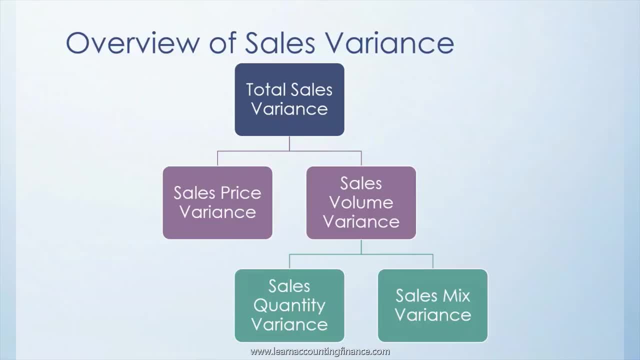 the change in percentage of each product in the total mix of your sales. We will take a look at this example in detail in the courses that follow. For now, it is good to know that the overall sales variance is divided into sales price and sales volume, and sales volume variance is further. 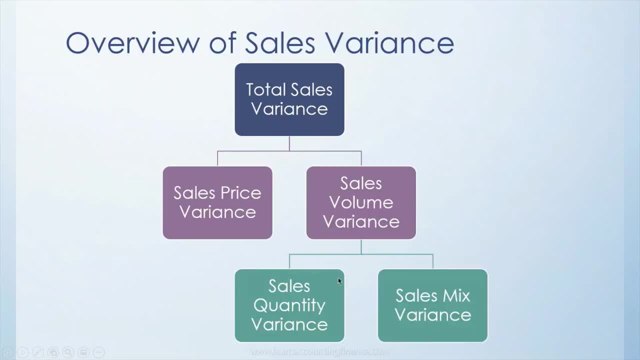 subdivided into quantity and sales mix variance, If you have market data available. the sales quantity variance is also further subdivided into market size and market share variance, But this is beyond the scope of this course For now. it is good to know that, if you understand. 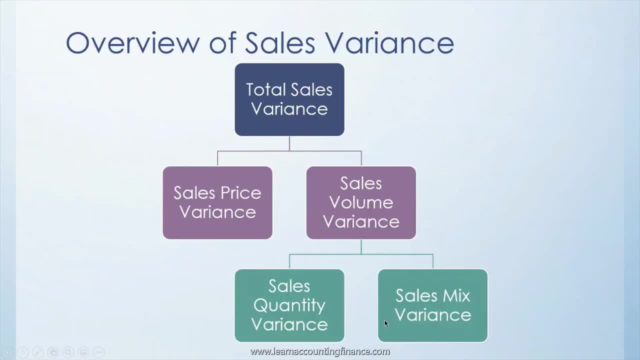 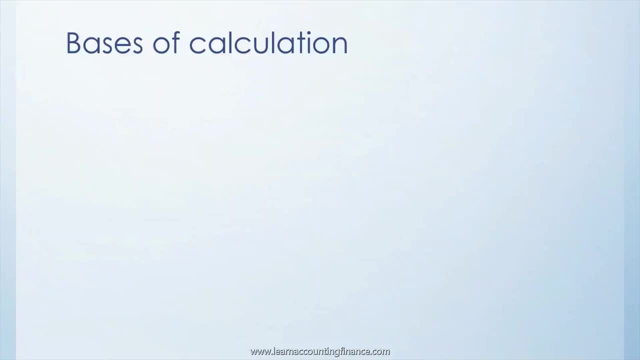 the difference between sales quantity variance and sales mix variance. you can also easily calculate market size and market share variances. An important question is: what is the basis of calculation that we use in calculating sales variances? The most commonly used basis are either profit, which could be your gross profit, or your contribution and selling. 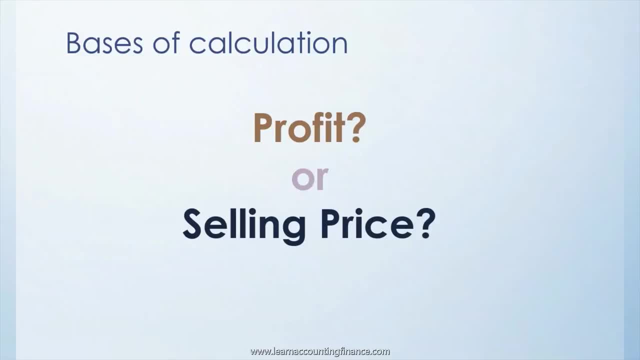 price, which is really the price of the product. The answer is: it really depends. If you are calculating the impact of sales variances on the profitability, you will use profit or contribution as the basis, And if you are using the impact of sales variances on the total sales, then you will. 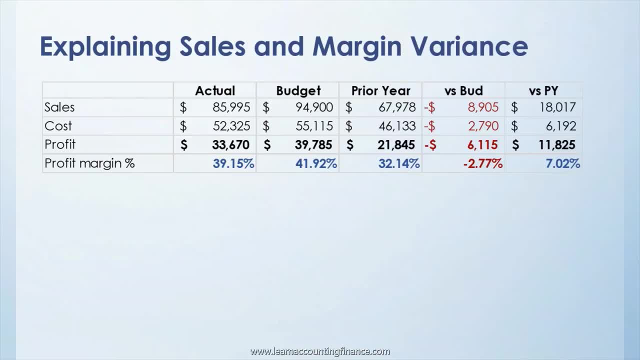 use selling price as your basis. Going back to our example, as you can see, the change in sales has impacted not only the sales dollars but also the profitability. So, for example, if we want to explain the change in actual versus budget of 8905, in order to explain this change into selling price. 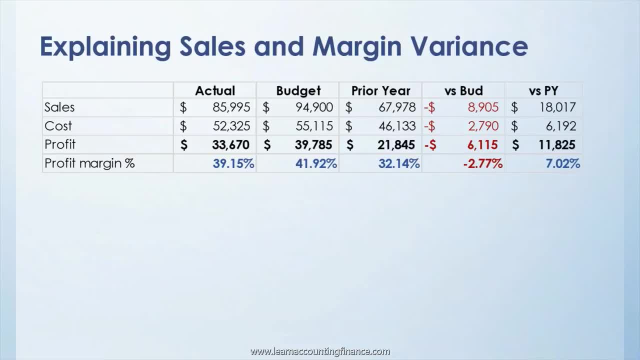 and quantity and mix, you will have to use selling price as your basis. But if you are trying to explain the profit change, which is $6,115 in this case, you will be using profit for your calculation. Just make a note of this information. this will be very useful and we will talk about it later. 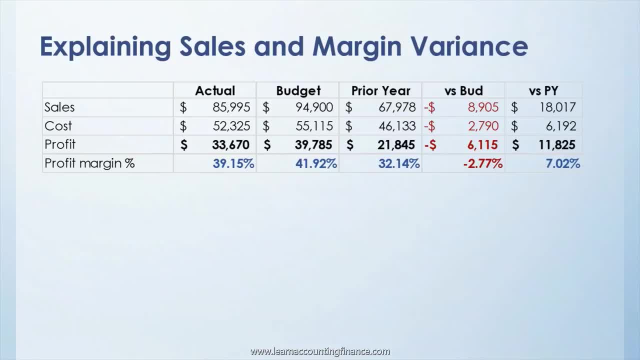 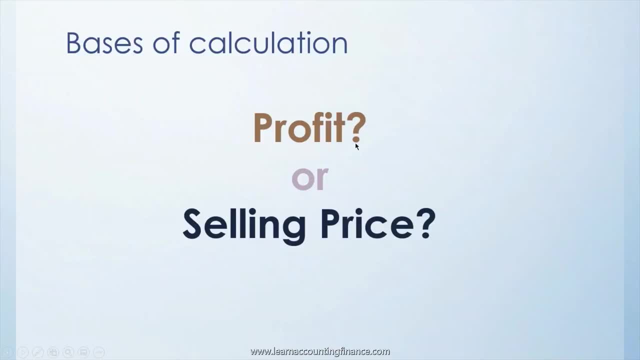 again, And once you go through the detailed calculation exercise, you will truly understand what I mean. For now, it is important to understand that sales variances can be calculated using either of those basis- profit or selling price. but they are each for a different purpose And you should. 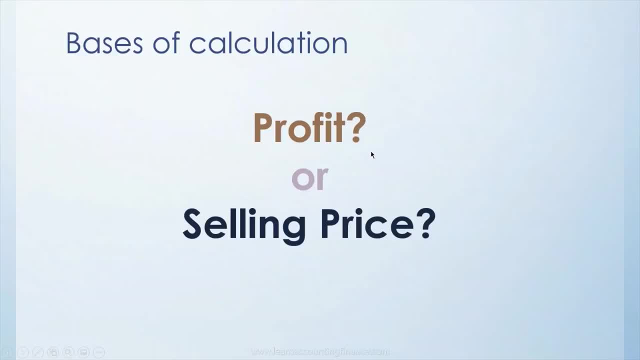 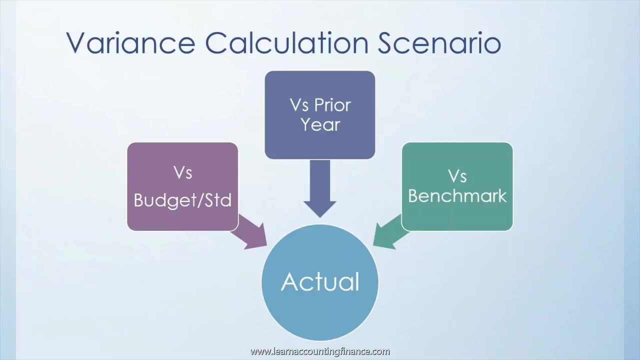 know what are you trying to explain in each case. Another important question is the variance calculation scenario. So let's say that you are using the variance calculation scenario, So really, what are you trying to calculate the variance? again, What happens most often is that you have actual results, So you have actual sales results. 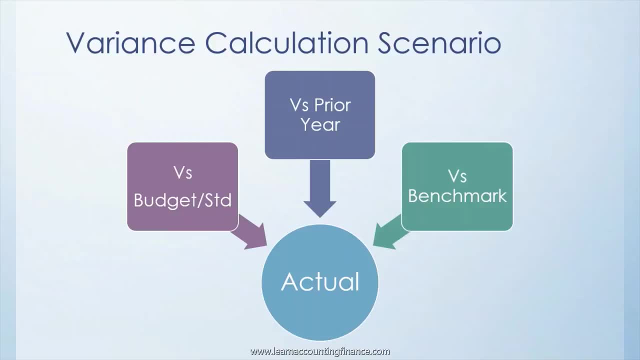 actual sales, actual profit, and then you are comparing this with another reference point. So you may be comparing your actual results versus budget or standard. if you are using standard costing, You may be comparing your actual results with prior year, which is last year. It could be prior month. also it could be prior. 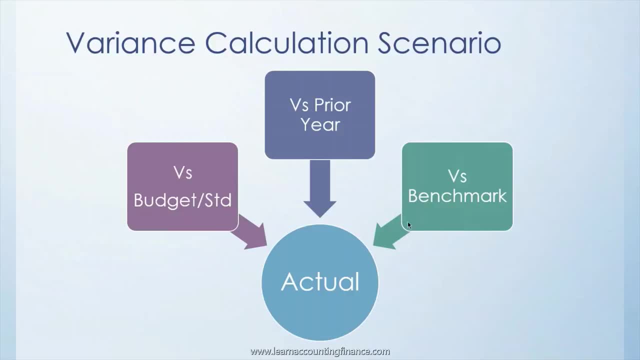 week really depends. and then also, you could be comparing your actual results versus a benchmark, which could be industry information or, you know, information related to a competitor. all of that does not matter. really, you can compare your actual results with anything. as we go through the detailed calculation, you will see that we can set up our Excel file in a way that we can. 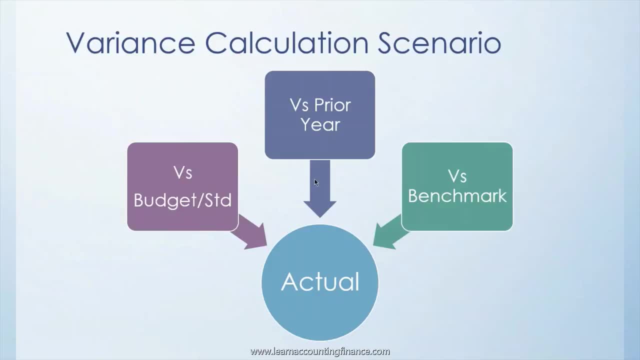 compare our actual results with budget last year or whatever other information we want to compare it with, and the calculation will work just fine. this will be the beauty of this course. once you have the files set up, it does not matter what is the scenario. what are you trying to compare the variances for the? 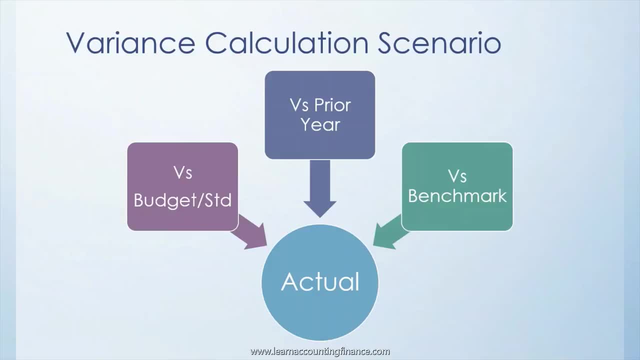 formulas will work, the calculation will work. it always have up-to-date variance analysis. however, most commonly, the two scenarios that we see most often is comparing your actual results versus budget or comparing your actual results versus prior year. in businesses, in organizations, management are really interested in knowing how did they? 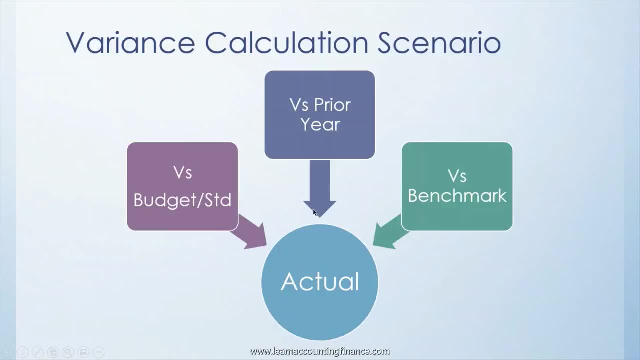 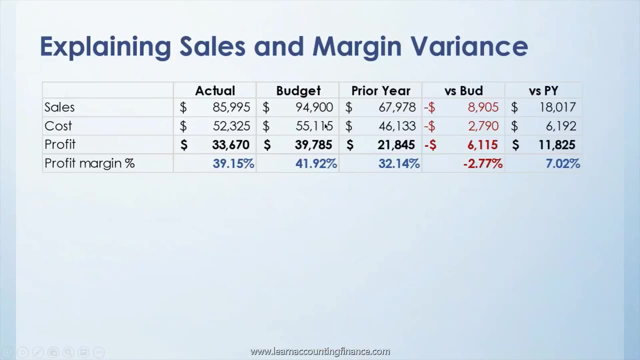 perform versus their budget or plan, and how did they perform versus prior year? in this course, though, we are only going to look at the two scenarios, which is actual versus budget and actual versus prior year, as you can see in this example, so we will not look at actual versus benchmark and any other scenarios, but, as 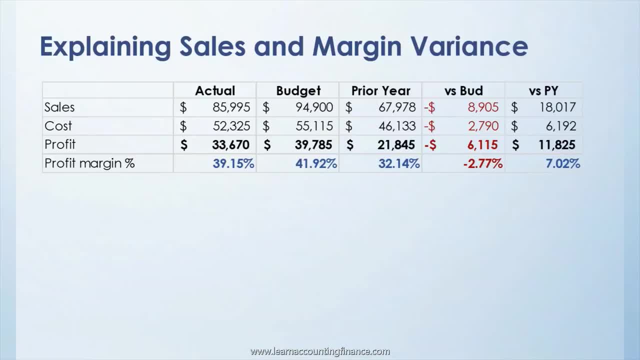 I mentioned. these are the most common scenarios. once you learn to calculate the impact of variances and variance analysis, once you learn to calculate the impact of variances and variance analysis against one scenario in this course, you will be able to use it against any other scenario. 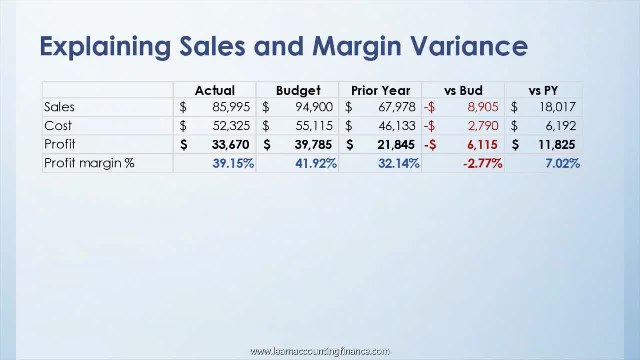 So that should not be a problem. I just want to highlight one more point here, and that is we are looking at the sales variances and the impact of sales variances on profit margin and overall profitability of a company. What we are not considering here in this course. 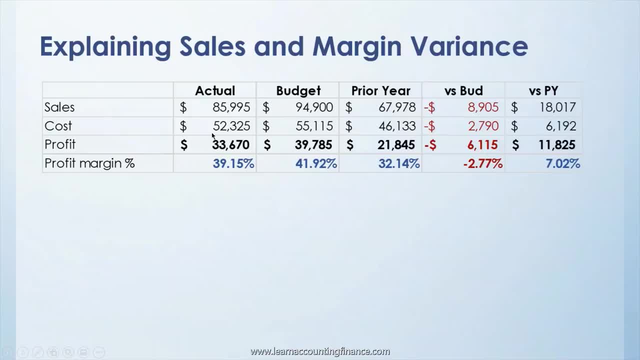 is the changes in costs, the impact of changes in costs. So variances related to changes in costs, for example, purchase price variance or material mixing variances, labor variances- We are not considering all of those variances for this course but, as you will see, 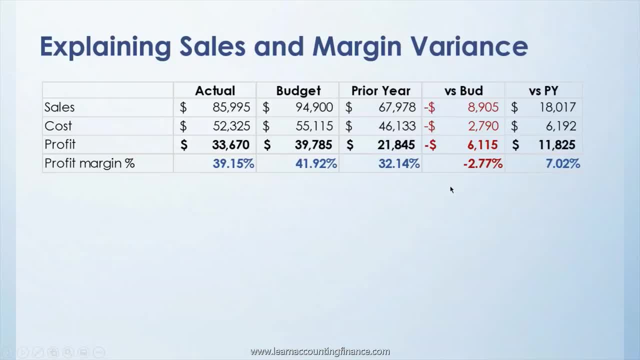 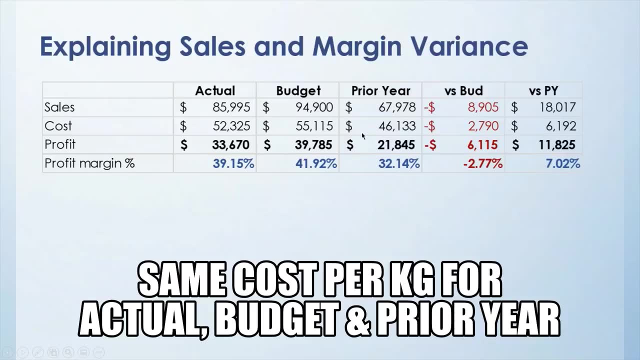 it does not matter if cost changes as well. For our example, for our scenario, we are not changing the costs between actual budget and prior year. The costs remain the same. The only changes are in the selling prices and quantities between these three scenarios. 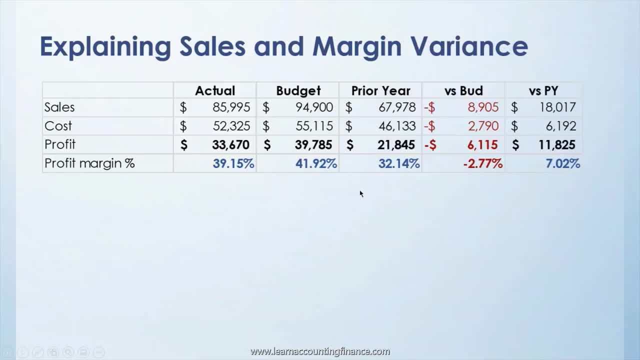 But once you go through the detailed exercise, you will notice that when you are calculating sales variances, it does not matter if there are changes in costs. but this is out of the scope of this course. Once you understand how to explain sales variance. 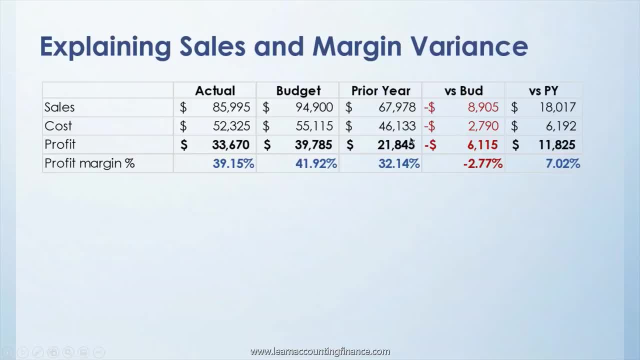 it will be very easy to explain the impact of cost variances as well, because this is the key point- This is where many students, many professionals struggle as well- is explaining the impact of variances in terms of dollars and in terms of profit margins. 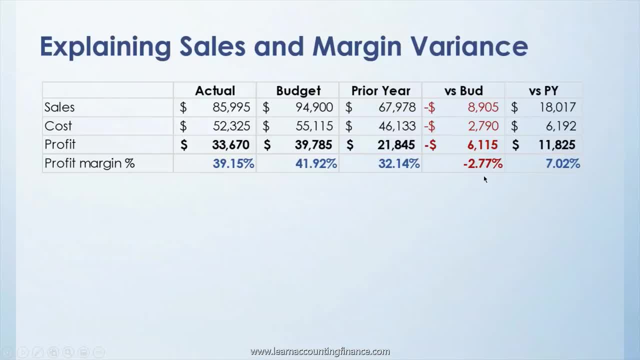 margin percentage changes. These are critical. These are questions that are asked every month, sometimes more frequently than that, because these are important questions that the business wants to know and should know, And that is what we are covering in this course. So this course is. 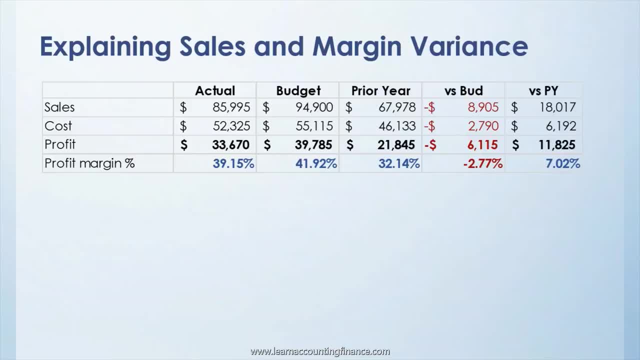 about sales variances and the impact of sales variances on the profitability. It does not cover costs but, as I said, when calculating sales variances it does not matter if there are changes in the cost, And we will take a look at that in detail once we go through the exercise. 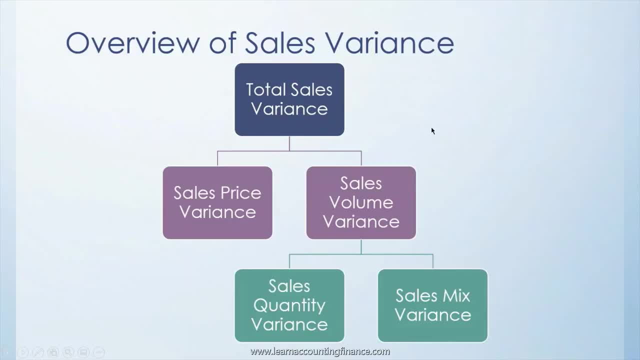 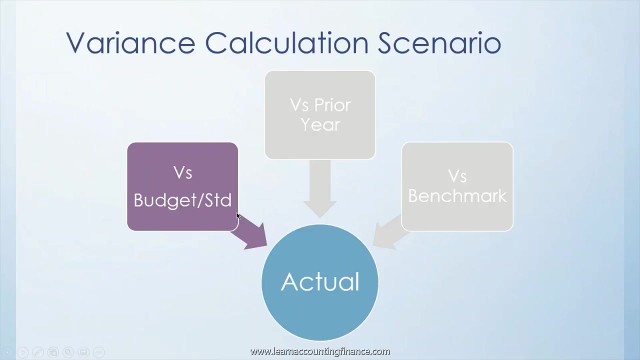 All right, now the exciting part. So, as you can see, this is the overview of our sales variances. We are going to start first of all with sales price variances. For our first exercise, we are going to take a look at the scenario which compares our actual results with our budget results. So, yes, 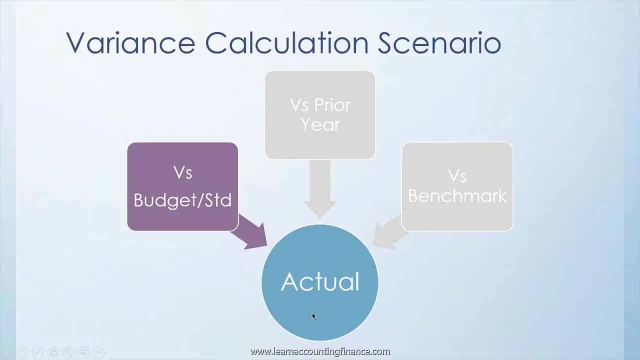 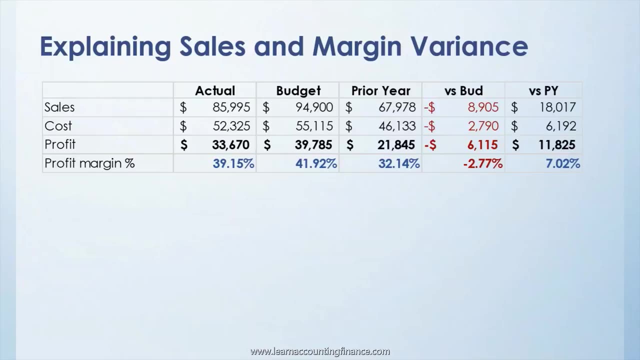 this will be sales price variance, comparing our actual results with budget results. Let's get right into it. So, going back to our example in the introduction section, we are actually going to solve this problem. We are going to use the same data, the same information and try to explain the 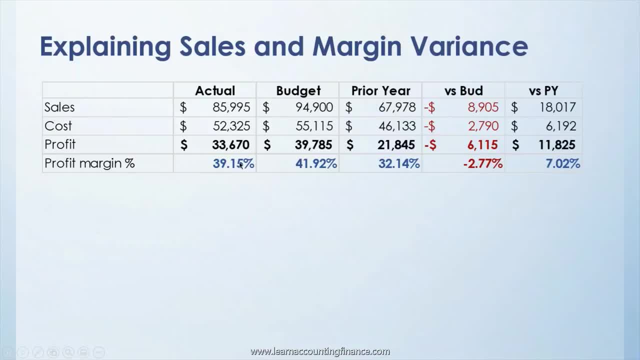 variances one by one. So, as you can see, our actual sales for the year are $85,995 versus budget of $94,900.. So there's a difference in sales of $8,905.. And we are going to take a look at. 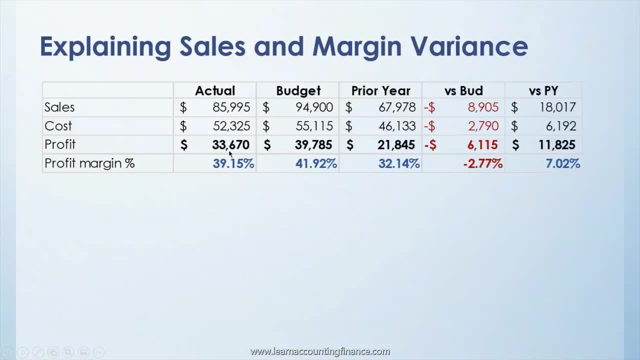 the profit. And if you look at the profit, your actual profit is $33,670 compared to a budgeted profit of $39,785, which gives us a difference of $6,115.. So we are trying to explain the $6,115. 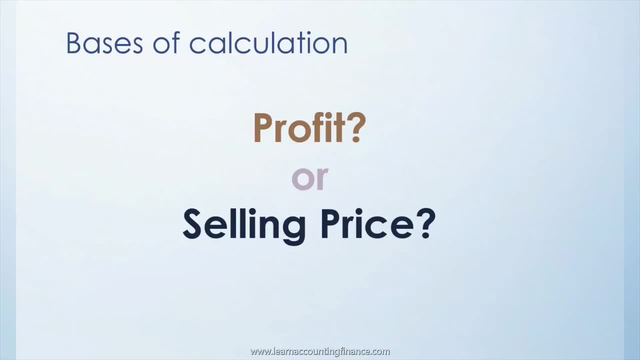 We are focusing on profit. You remember our slide where we said we could either choose profit or selling price as the basis of calculation. Most often what businesses are really interested in is in their profit, So we will start with profit as our basis of calculation. So if I put our slide information on our slide next to the 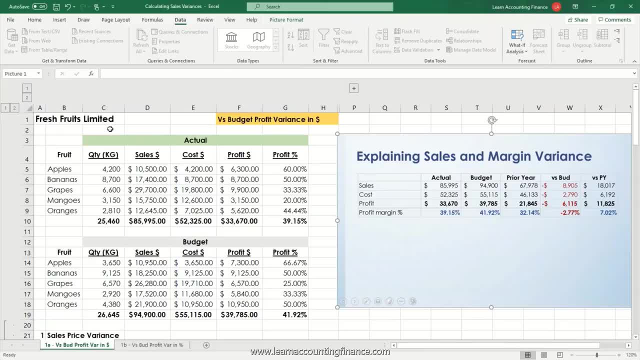 data in Excel sheet. you will see that, our Excel sheet, you know. you will see that this information is actually related to Fresh Fruits Limited And the sales and profit that you see over there is really related to these five different types of products. So we are going to take a look at the 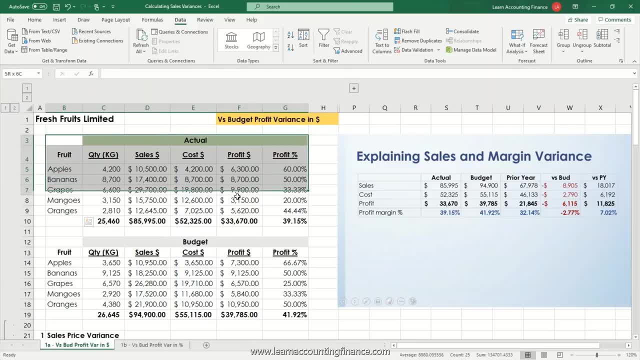 different types of fruits that the company sells. So we have actual data in this section and we have budget data in this section And you can actually trace and you can see the numbers do match. So, for example, the sales for the actual sales for Fresh Fruits Limited is $85,995.. You see this number. 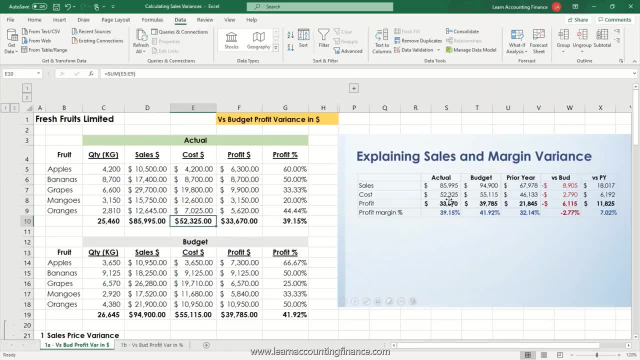 matching here And then, similarly, cost is $52,325.. And profit is $33,670.. You can see the profit margin percentage. That's $39.15.. Similarly, you can see the data for budget matches as well. And once we get to the 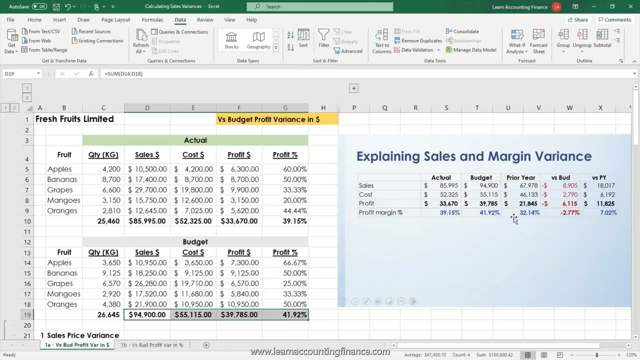 priority information, you will see that that information will also agree. So we are using the example we showed, the summary we showed in the first place, And we are going to explain each of these variances one by one. So let's take a look at the detail that we have here. If you look at 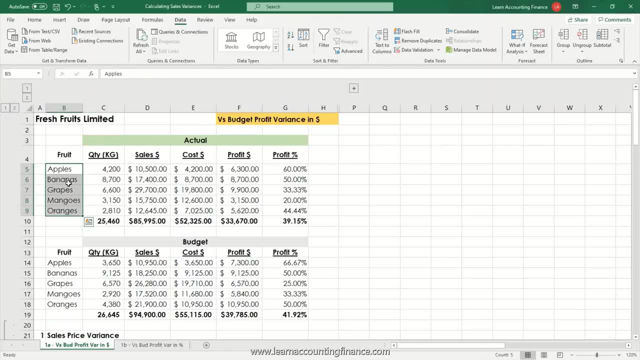 Fresh Fruits Limited. they sell five different fruits: apples, bananas, grapes, mangoes and oranges. You have the quantity sold. This is the actual quantity. Again, this section is actual section. So you have the quantity sold for each fruit, you have the sales dollars, you have the cost and you have the 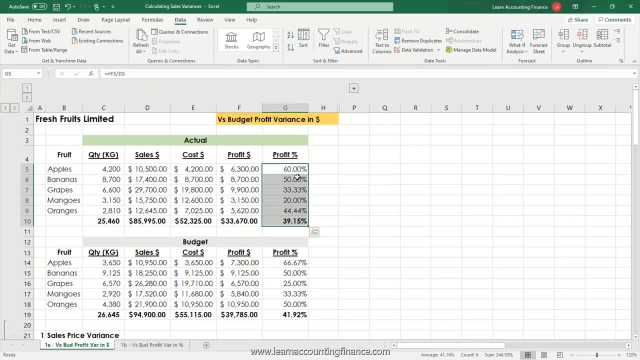 profit dollars, And on the right side you also see the profit percentage or the profit margin. Similarly, you have the same information related to budget for that here. I have made a few calculations for you already, which should be very simple. What I've done is really calculate price. 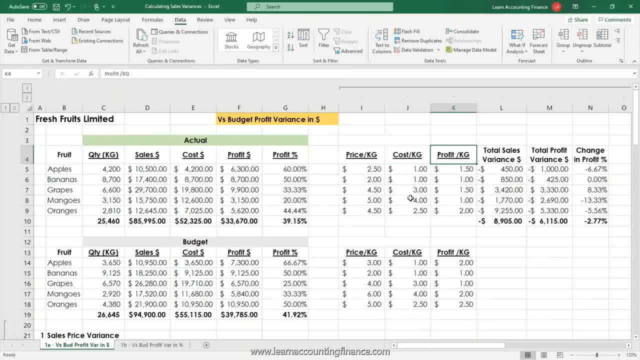 per kg, cost per kg and profit per kg. And just as an example, the price per kg is really your sales dollars divided by the quantity of kg sold for the fruit and similarly cost and profit. So what we do, we see if you compare actual 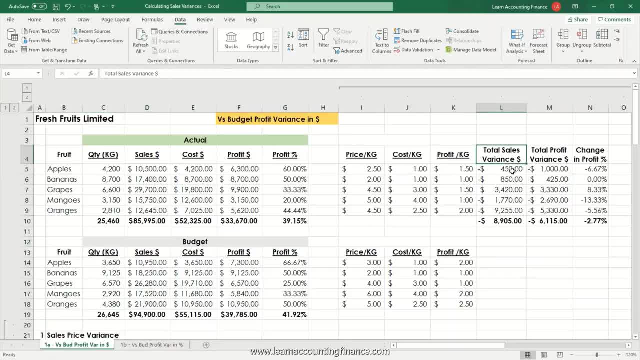 results. the budget is that you have total variance in sales dollars, which is $450 for apples all the way through to oranges and oranges. However, the net profit money- this is half of the revenue- $40,000 and that is $355 per kg. So our profit is $3375 per kg. 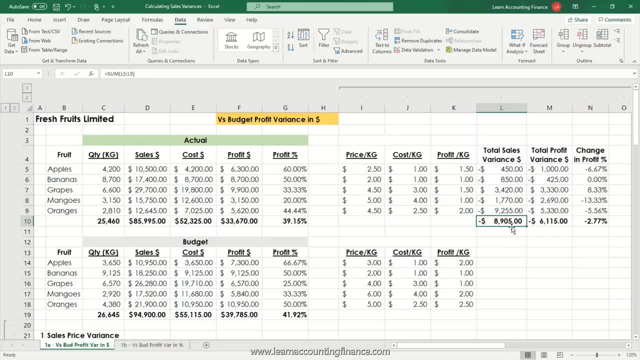 and you can see this total number of 8,905 should look familiar now, because we have seen that in our example. Also, 6,115, which is the change in profit, should look familiar. and then, of course, the 2.77 percent are the drop in margin versus budget. okay, or you can say the gap in margin. 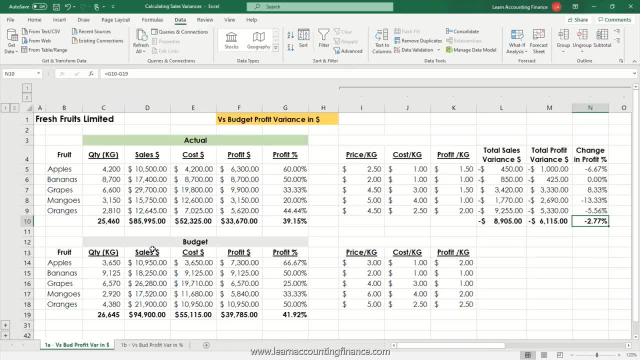 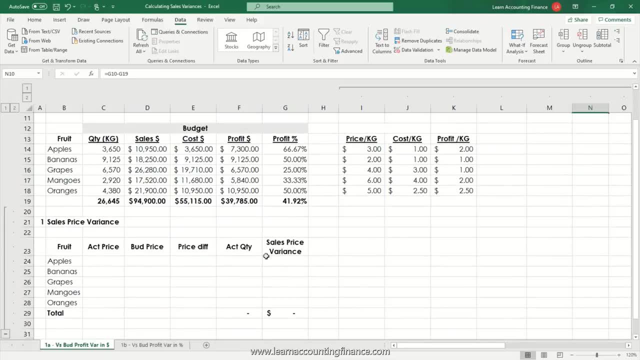 versus budget. So now we take a look at our first variance, which is the sales price variance. Let me expand the box here. I have created a quick table. So sales price variance, as we mentioned, is the difference between your actual price and budget price, in this case, If it was prior year. 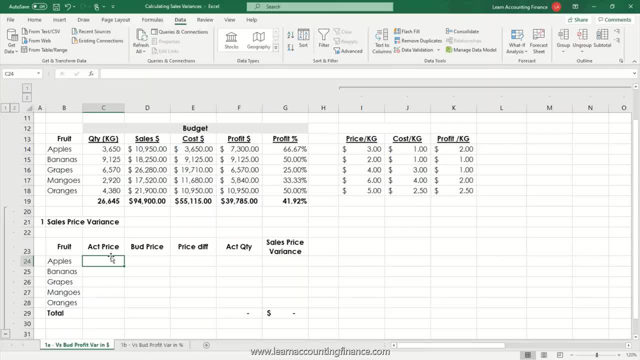 it would have been prior year price, but now we are dealing with budget. So actual price versus budget price will give you the price difference and then you will look at your actual quantity. and that means if you multiply your price difference with your actual quantity, you'll. 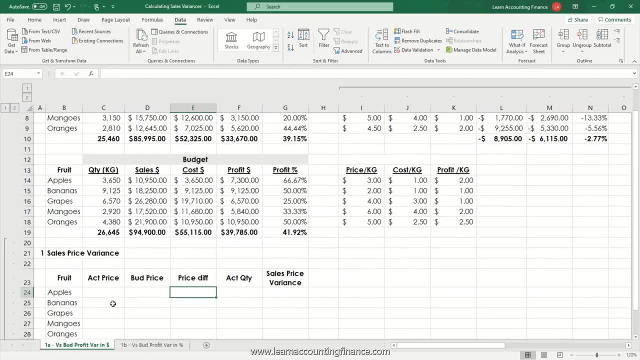 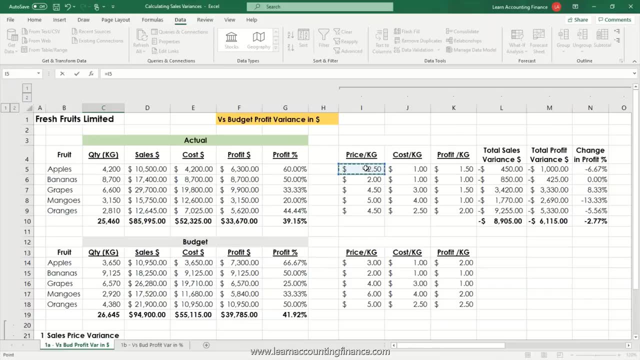 get your sales price variance. So let's do that quickly. We have actual price here. I'm gonna just link it to the prices that we have calculated. So this way, even if the numbers change, even if the scenarios change, our calculation will always work. 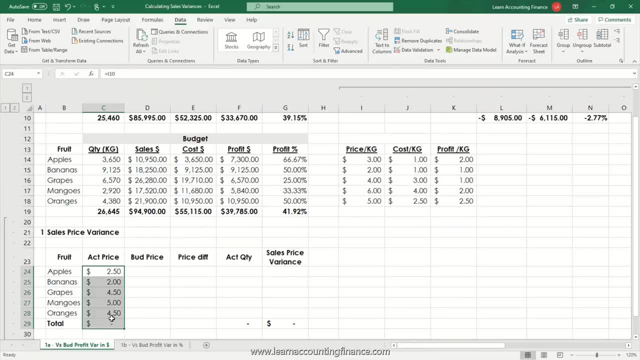 So this is the purpose behind linking all of them. Similarly, we can link the budget price, which is right here, and you can already start seeing some differences in the prices, but you can also link the budget price with a discount, so that's pretty easy and easy. 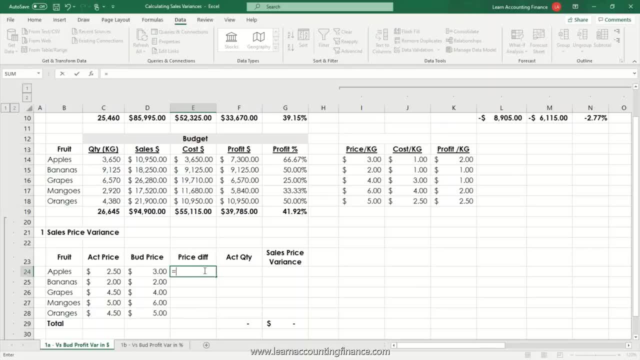 but you can also link the budget price with a discount, so that's pretty easy and easy calculate. when you are calculate, when, when you are calculating, what is important is that you should always um calculate the difference, starting with your actual price. so actual price goes in first. 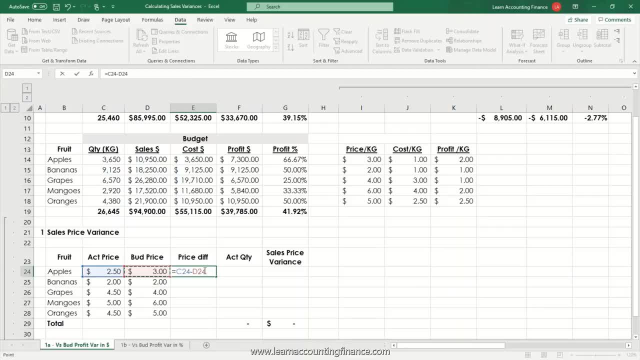 and then budget price goes in second, and the reason for this is you want to show any drop or any unfavorable variances as negative amounts. right makes sense, right? um, unfavorable is a negative sign. so in this case, our price versus budget is lower, which is, as you can see, the 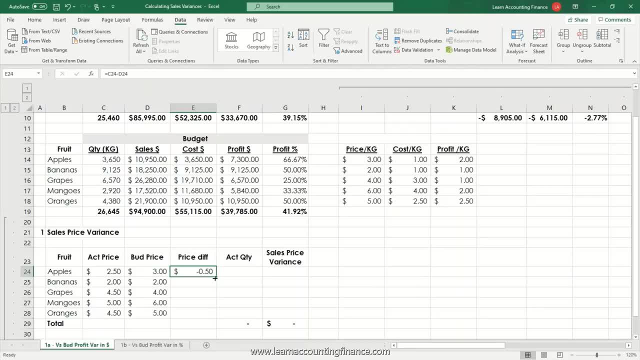 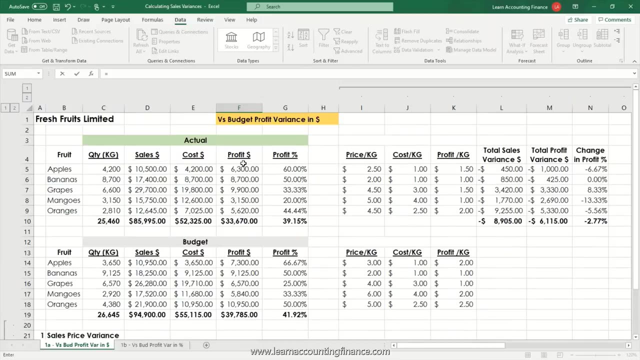 budget was three dollars, or actual price is 2.5, so 50 cents lower, and all we do is just copy it down. drag this down and you can see all the prices. price differences are calculated, and then for this calculation we will consider actual quantity sold, which we already have up here in the example. 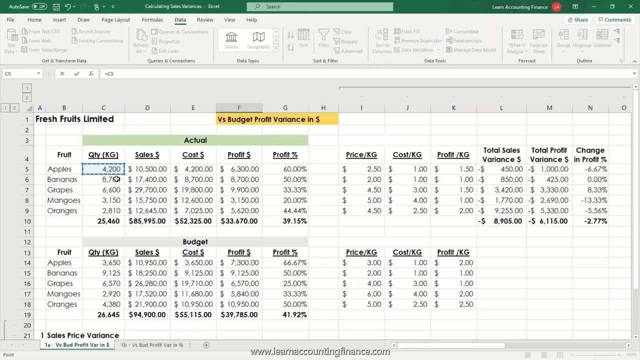 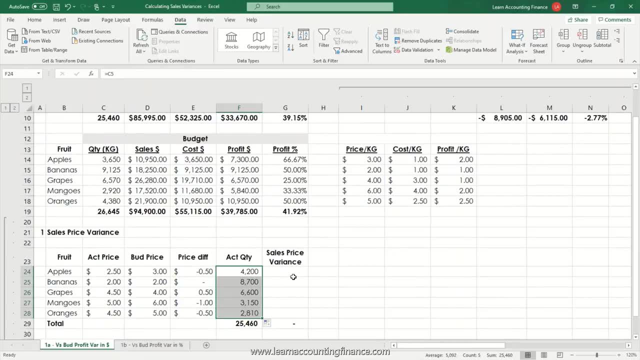 so for apples, we reference it to apple, which is 4200 kgs, and as you drag it down you have all the quantities and the sales price variance simply is the quantity times your price difference. so, as you can see, 2 100 for apples. this is unfavorable ratings. 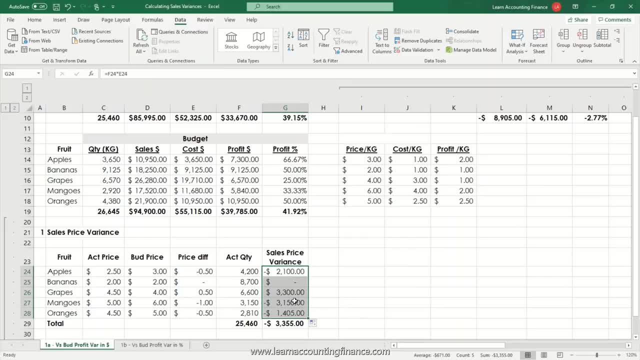 if i drag it down, you will see um. the total variance is 3 355 dollars. uh, you can see. there's no price variance for bananas because the price did not flip lists dead. the sales price is the same as our plates, so there's no variance for bananas. 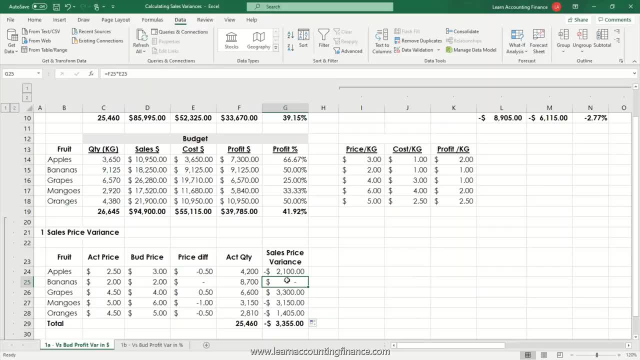 it is non-variable and the actual price is the same as the price. so, in other words, blow around long period of time. uh, the actual price is the same as budget price. so there's no unfavorable or favorable variance there. then variance is zero. so that's it. we have calculated. 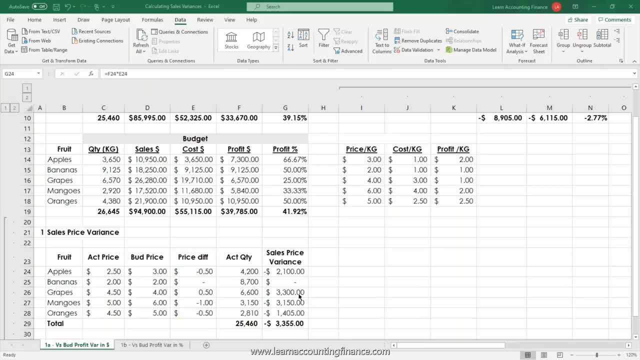 our sales price variance. already now you can see our total variance is 3-1355, but there are a few, So this one grapes. this food is actually helping us in our total sales variances. On the other hand, for bananas we have no variance because the price did not change. 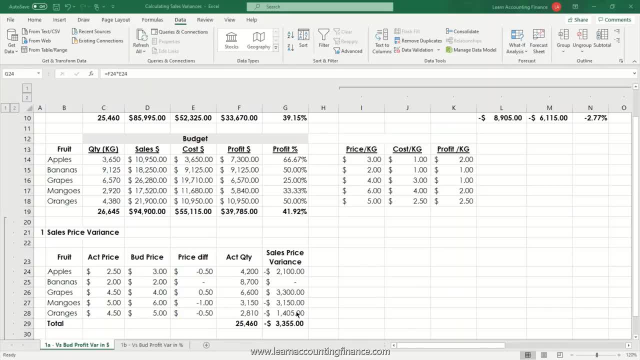 Then apples, mangoes and oranges, we see unfavorable sales price variance because the actual price is lower than the budget price. An important point I want to make here is that again we are looking at the impact of change in sales variance on the profitability. 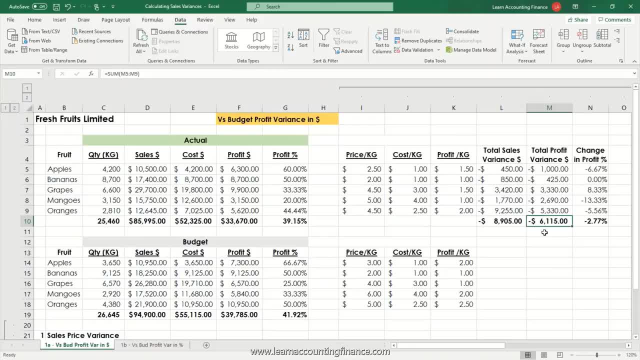 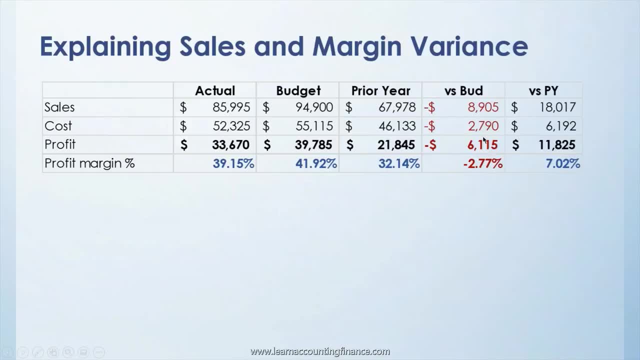 So in this case we are going to try and explain the 6,115.. If you go back to the example, this example here, you can see that the actual profit is under budget by 6,115.. But when it comes to price variance, all of the price variance impacts of a profit right. 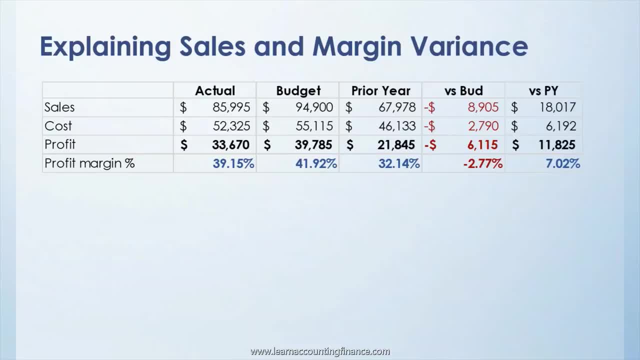 Because any change in the price will directly flow through to the profit. What is profit? Profit is your sales minus cost. If cost does not change and your sales changes or your selling price changes, all of that will be a direct pass through to your profit. 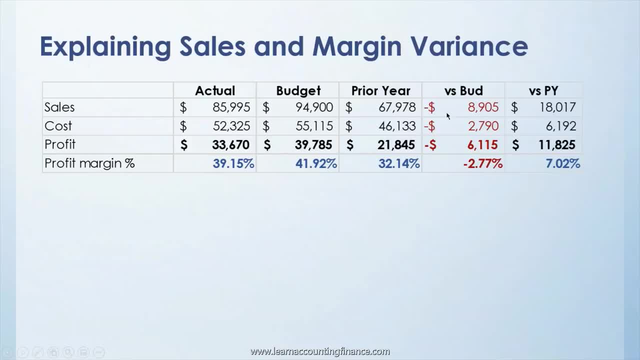 So your sales variance Is the same in terms of dollars and profit right. So impact for both sales dollars- 8,905, and profit dollars is the same. You calculate it in the same way as far as sales price variance is concerned. 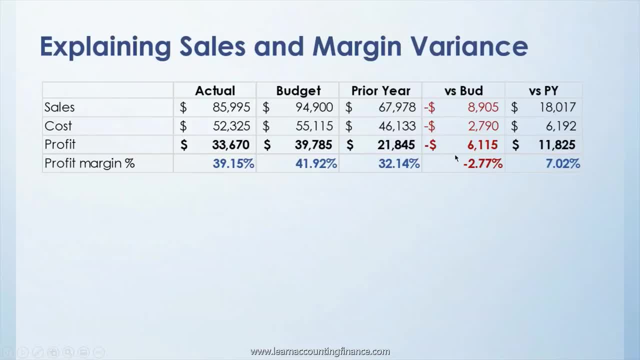 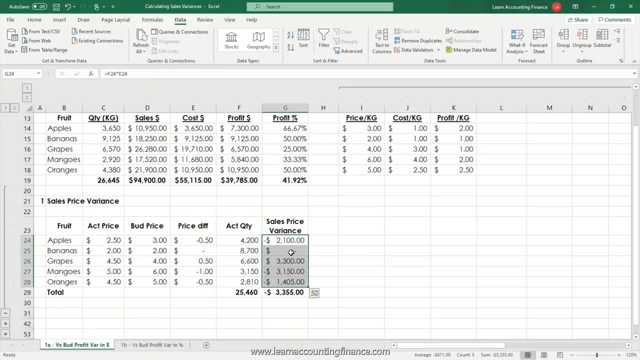 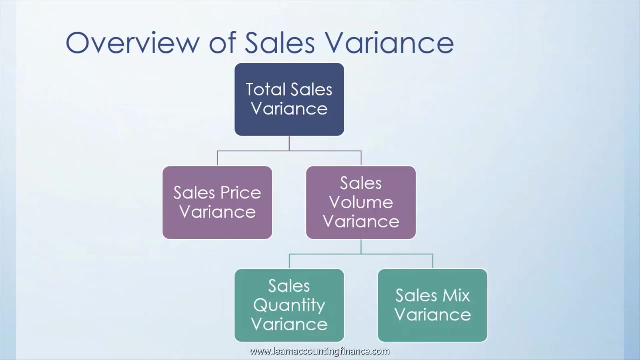 It is not the same, though, for sales volume variance, which we'll get to in a minute, But for now, we have calculated the sales price variance, and let's move to the next step. Okay, Now we are going to take a look at our second variance, which is the sales volume variance. 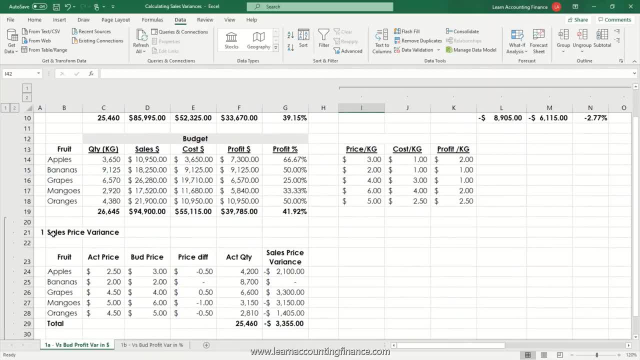 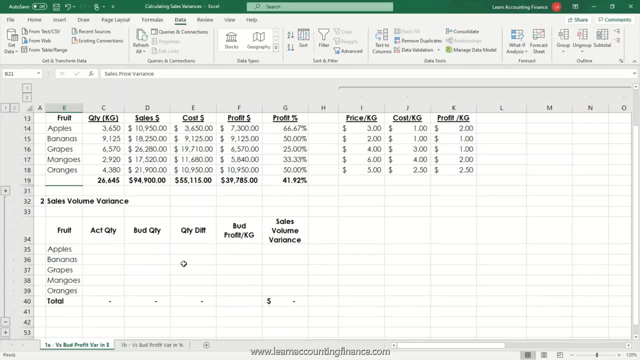 So, going back to our example, we have already finished the calculation of sales price variance. Let's collapse this and let's open up sales volume variance. So what is sales volume variance? Sales volume variance is really the difference between actual and budgeted quantity. 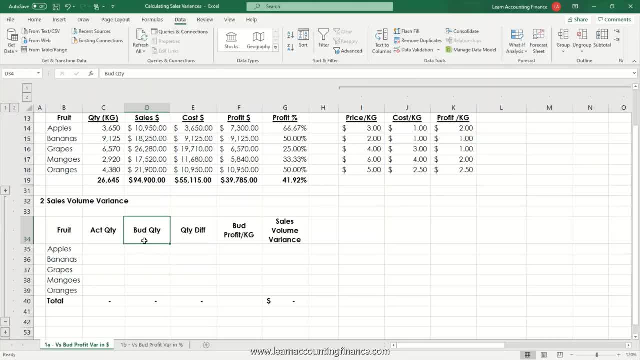 As price variance was the difference between actual and budgeted price. sales volume variance is simply the difference between actual and budgeted quantity. Let's calculate that and then we'll discuss this further, So we can simply again link our actual quantity based on the data that we already have. 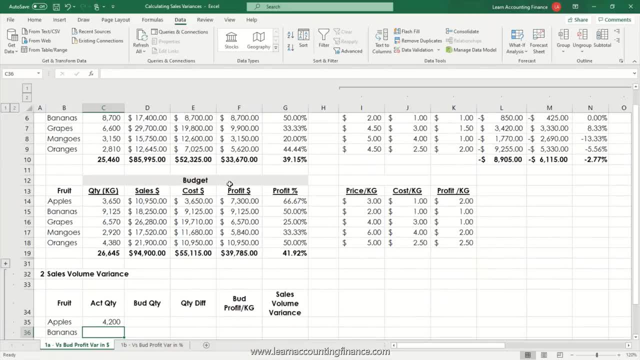 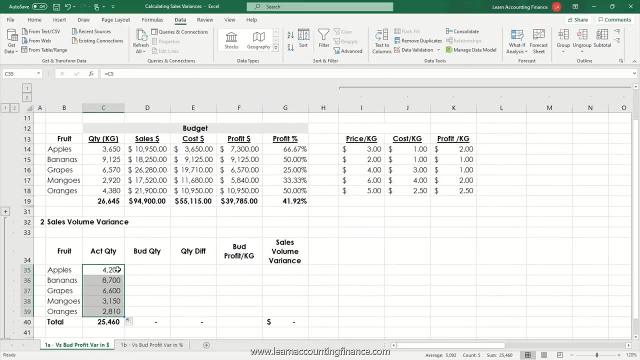 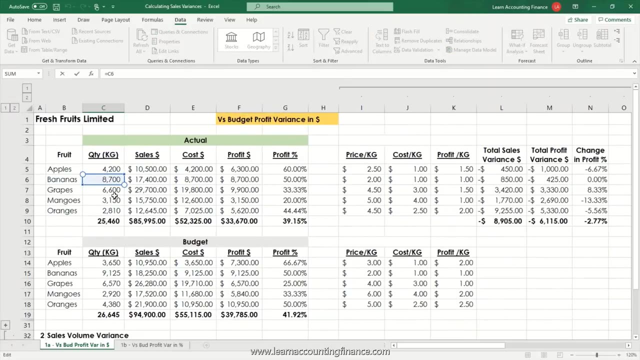 So we know our actual quantity is here. So after linking I can just drag down. We can also use copy and paste to keep the links there. So, as you can see, for bananas the link is to the cell reference C6. And similarly we have copied all the actual quantities down. 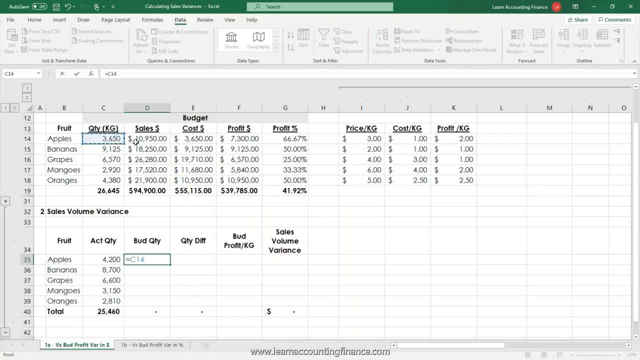 For budget. we will do the same thing, As you can see: budget quantity by fruit or byproduct And this is our budget quantity. Now, again, we are going to calculate quantity difference And if you recall from our previous session I said we will use 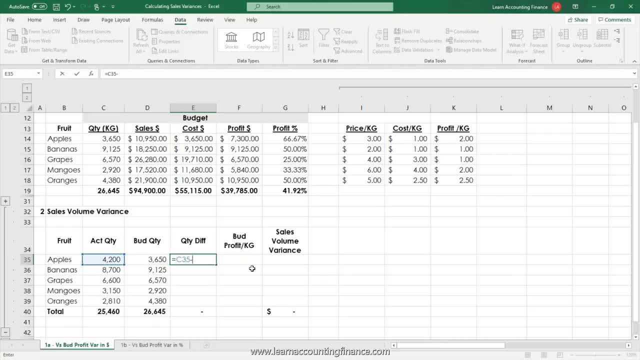 we'll always use the actual quantity or actual prices first and then budget quantity or budget prices Second, So you can see the difference here. As an example, you can see what actual apples sold is 550 kgs more than what was budgeted. 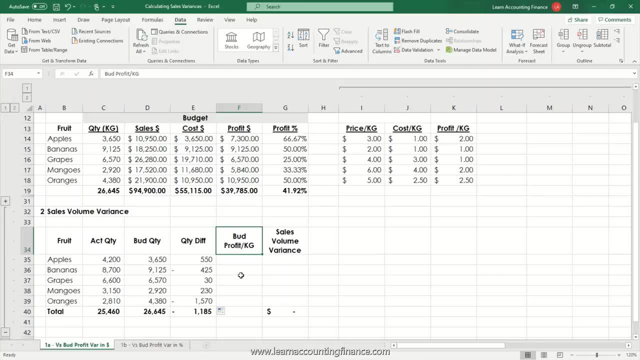 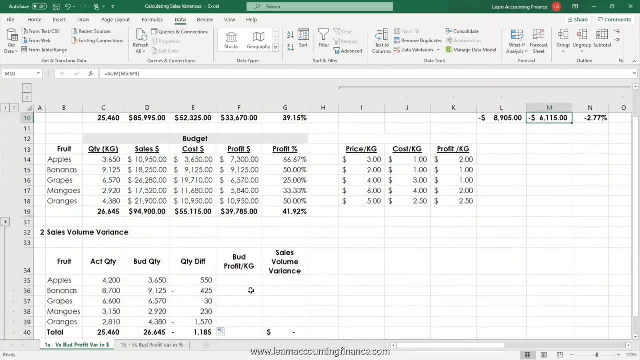 This is where the question comes in, that what is the basis of calculation you are using? We could have used selling price, But remember, we are trying to explain the change in profit, the 6,115.. So if we are trying to explain the change in profit, we will be using budgeted. 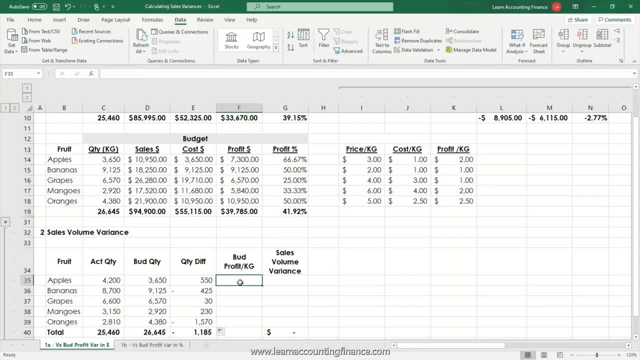 not actual profit per kg. And one more thing here is that we are using budgeted profit, not actual profit per kg, And, if you recall from one of our earlier sessions, I mentioned that we are not covering the changes in cost or cost variances here. 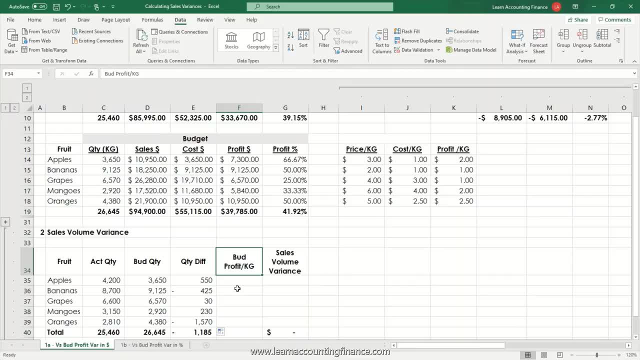 But this is the proof where it does not matter whether there is a change in cost or not, because we will always be using in our calculation, we will always be using the budgeted profit and not actual profit per kg, Even when we are comparing with prior year or any other benchmark. 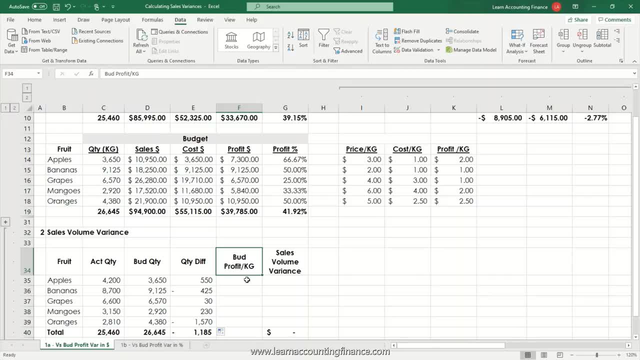 if, for example, we are comparing with prior year, we are going to use prior year profit per kg, not actual, for this year, And similarly for benchmark, we'll be using the benchmark profit per kg Right. So it does not matter if the cost changed from our reference point to our actual. 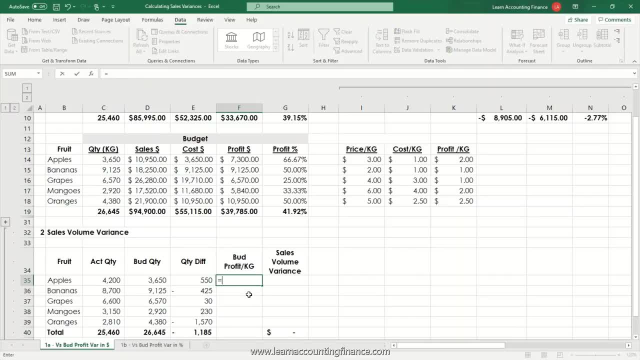 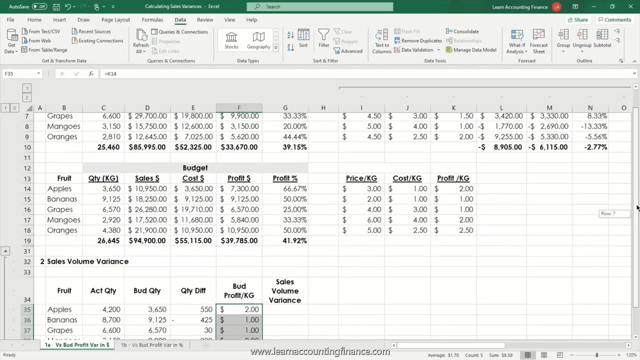 So in this case we already have the budgeted profit per kg. Again, I'm going to Simply link it. You can see, this is the budget section and we have budgeted profit here, And you can copy this down and just to just to highlight one more point or just. 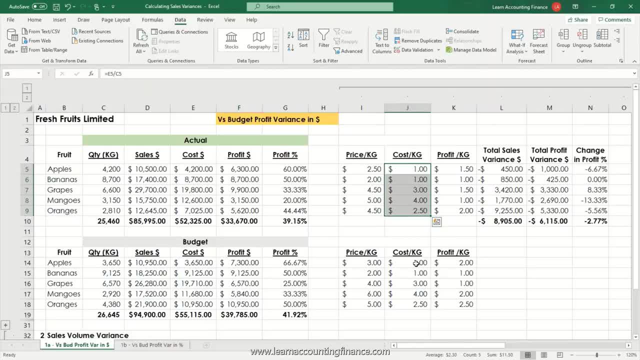 to confirm: as I said, we are not going to see any changes in cost per kg, So we are not seeing any variances in the cost. Our actual cost per kg is the same as our budgeted cost per kg. The only difference is the actual quantity changes, which results in a different 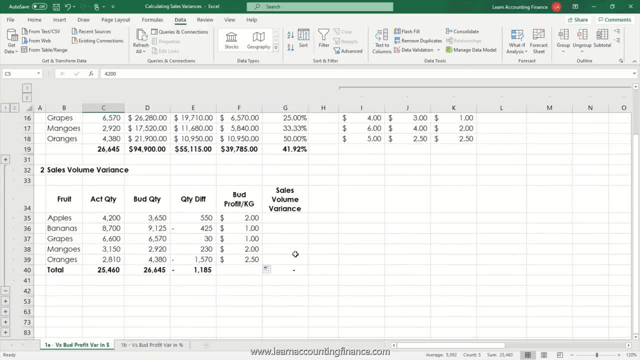 cost between actual and budget and budget. OK, so, going back to our sales volume variance, we have now almost everything we need. we have the budgeted profit, we have the quantity difference And again, sales volume variance will simply be a multiplication of our budgeted profit and our quantity. 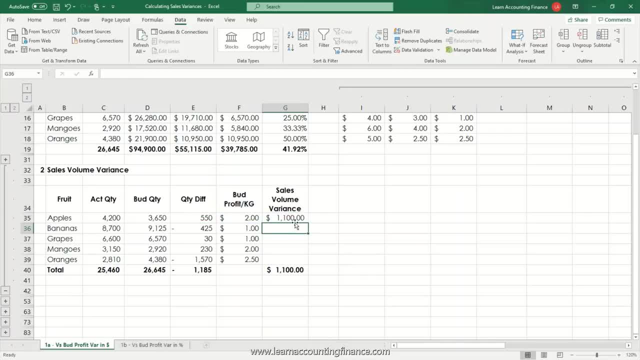 And our difference in quantities. So again, I'm going to drag this down And you see, our total sales volume variance is two thousand seven hundred and sixty. Now, at this point you should do a check If you are at this point in your calculation. 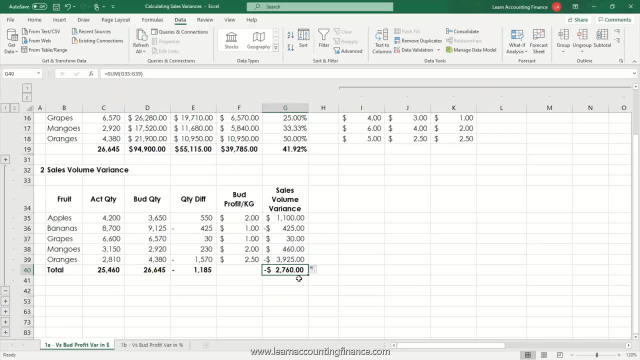 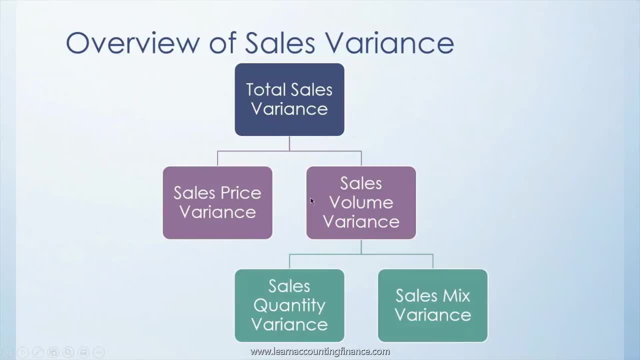 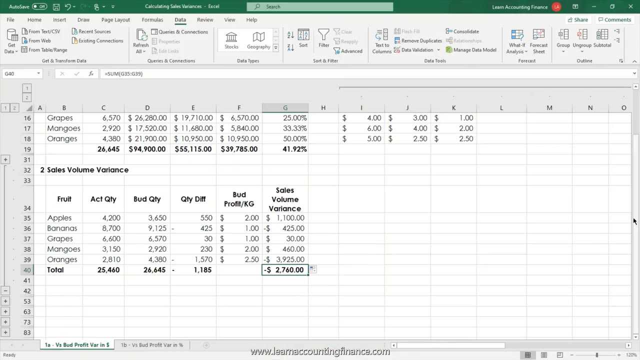 you should do your first check, which is going back to our sales overview. As you can see, your total sales variance is the sum of your sales price variance and your sales volume variance. So if I add the two variances that we just calculated, that should actually match. 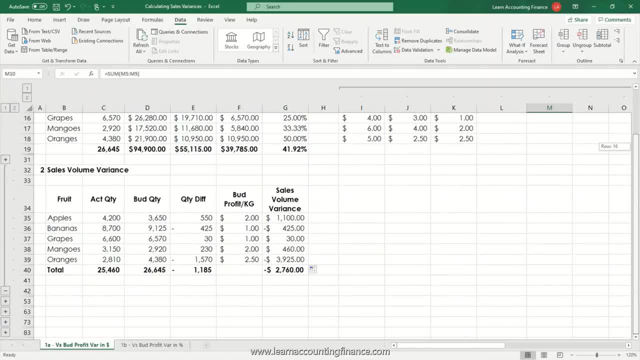 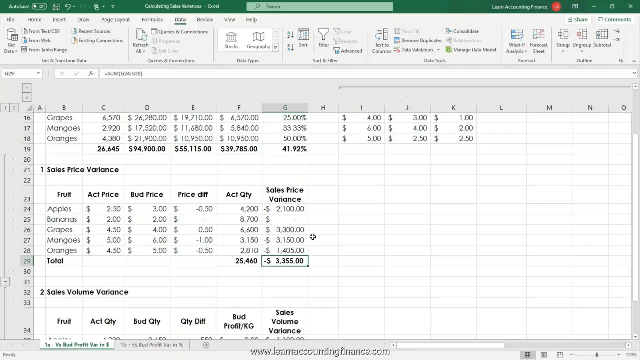 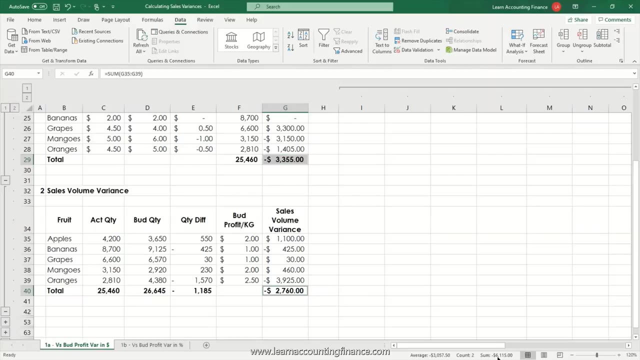 our total profit variance. Let's see if it works. So I'm going to expand our sales price variance And if I just select on this cell, which is the total sales price variance, scroll down, press control key and press and select this button. 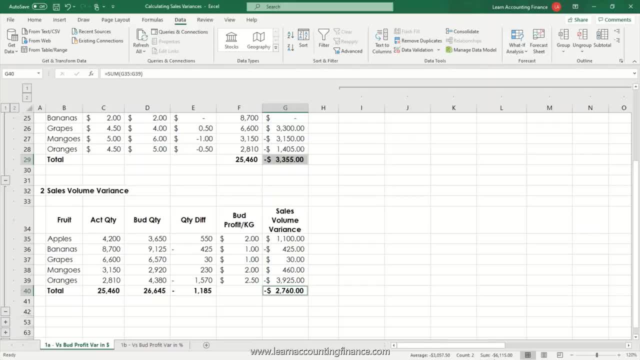 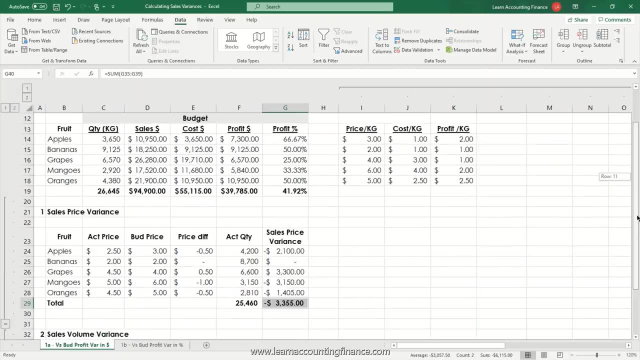 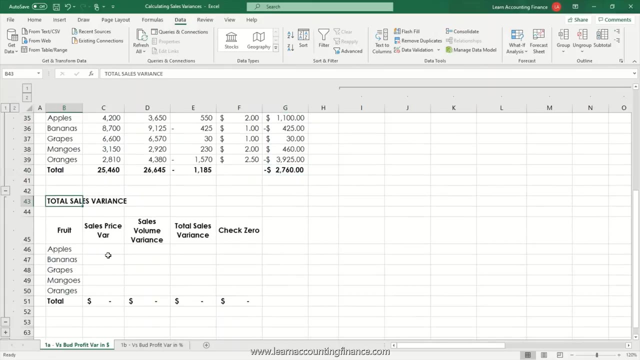 Exactly. You can see here in Excel, the sum is six thousand one hundred and fifteen dollars, which matches exactly the number we are trying to explain. So I'm going to Let's do a quick reconciliation here. This is the total sales variance. 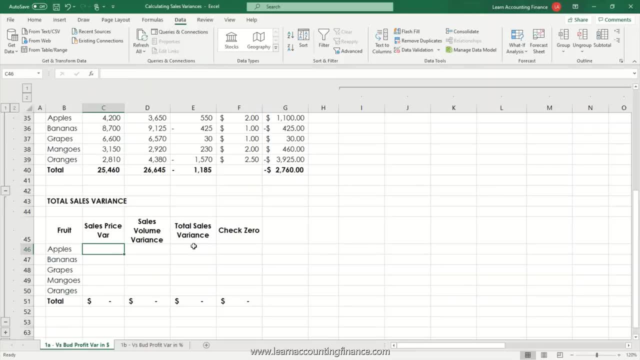 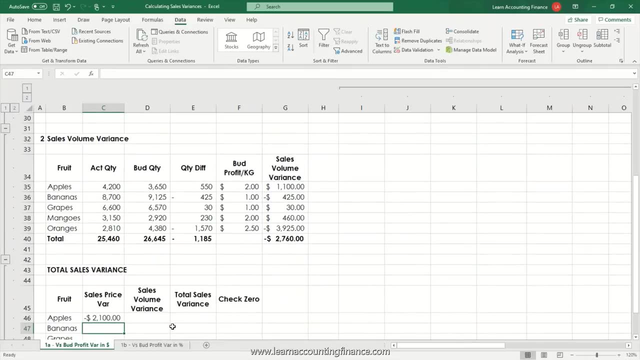 We know by fruit what is the sales price variance and sales volume variance. So if I look at sales price, we just calculated it right here. So like this: if you look at sales volume, we calculated it here And the total of the variance is this. 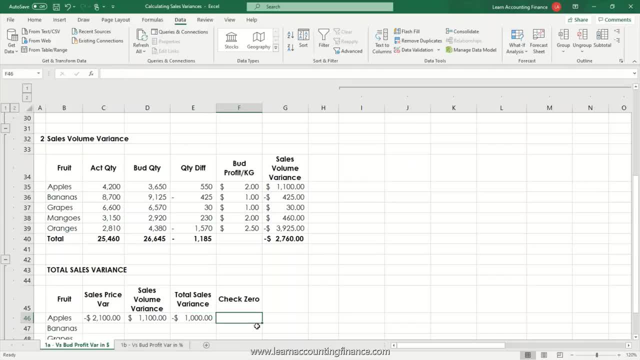 Sum of the two. Right, And we can also check This now, so we can check this against our original data. So if I take a look at this, this cell total variances minus, if I scroll up and look at the data here, 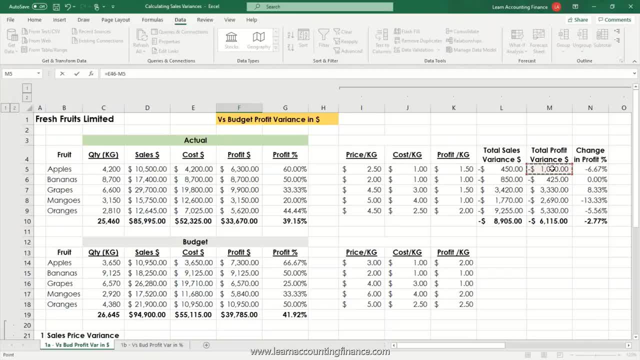 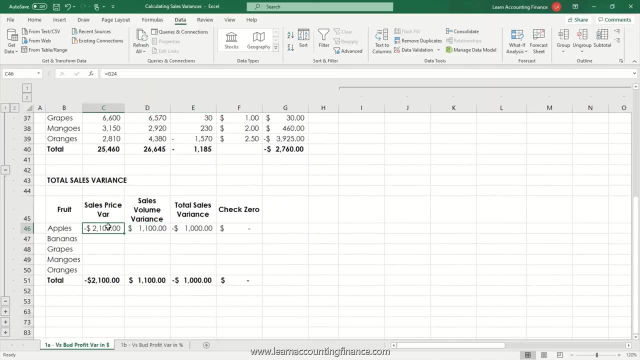 you see here this was calculated based on actual and budget data And this matches exactly. if I select all of this, Yeah, you can copy one cell at a time, or you can copy multiple cells at a time. So I select all four columns and then I drag them down. 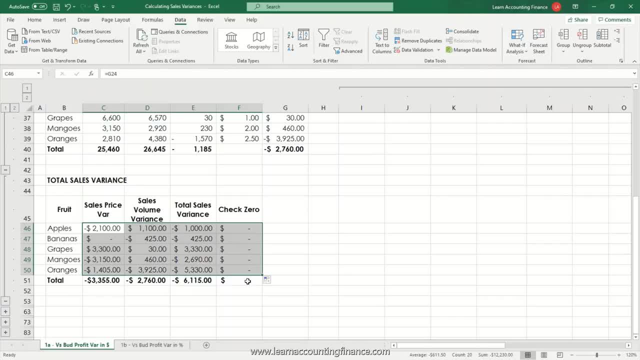 This will copy all the formulas and you can see the total check is zero, which means all of our variances are calculated accurately. Now you can see in a snapshot. you can quickly see what's causing the variances. Overall it's six thousand one hundred and fifteen. 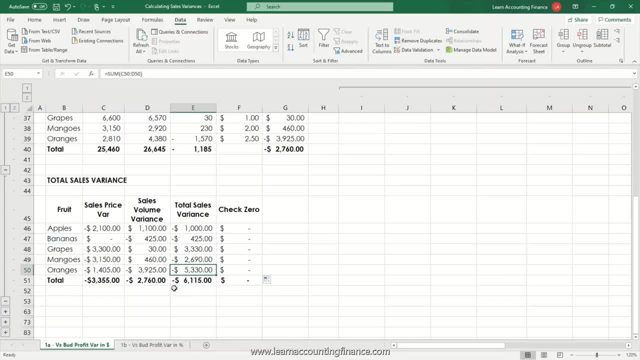 The biggest one is coming from oranges, And even within oranges you can say it's really volume. Right, That's three thousand nine hundred and twenty five dollars that are coming from volume. There is a favorable variance from grapes, mostly from the price. 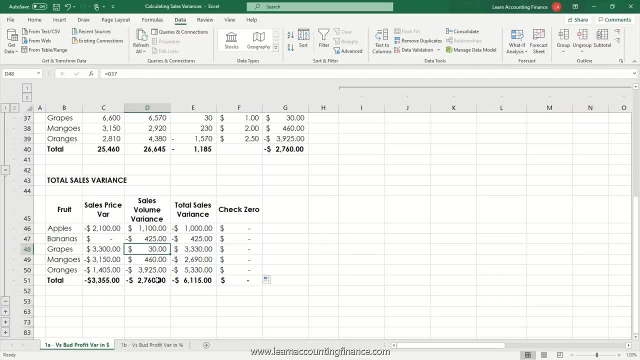 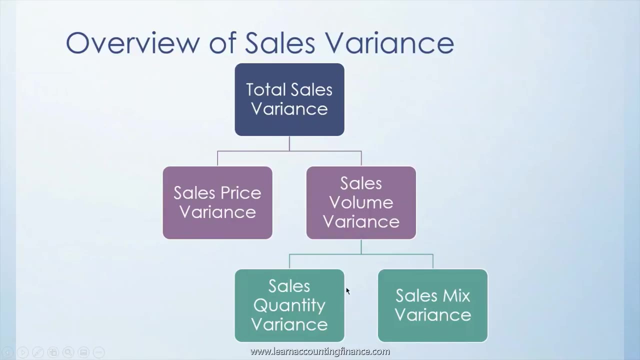 the price increase and to some extent from volume also because the quantity increased. But we have not fully understood volume variance yet And that's why in the overview of sales variance you see that sales volume variance is further subdivided into sales mix and sales quantity variance. 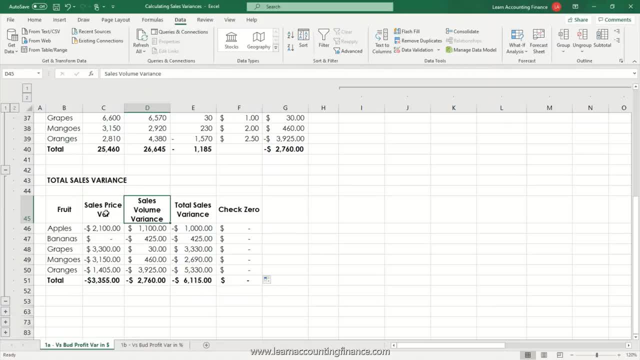 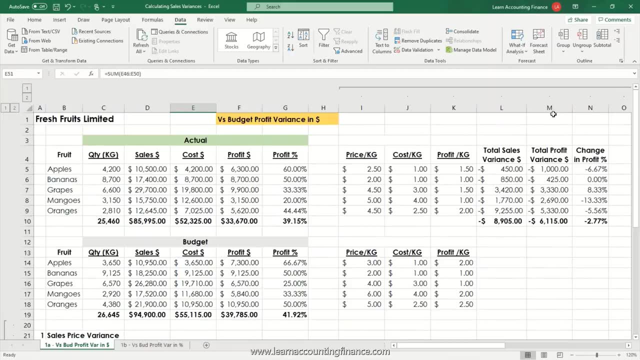 For the time being. we know that we have explained our sales price and sales volume variance, which is six thousand one hundred and fifteen. just to reinforce the point, Remember we were trying to explain variance in profit. We were not trying to explain variance in sales dollar at this point, although we can. 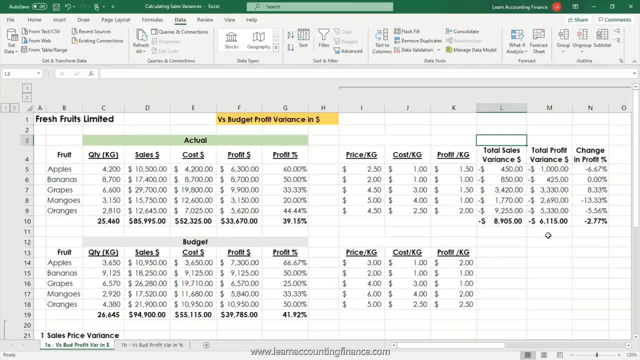 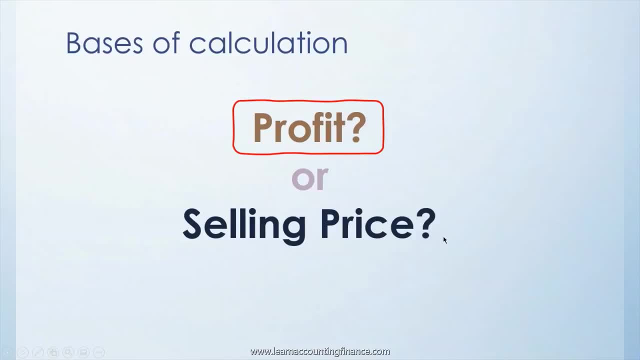 The only key difference between the two would be: what is the basis of calculation? And in the basis of calculation we said we are going to use profit as a basis. Had we used selling price as the basis, we would have been able to explain eight thousand nine hundred and five. 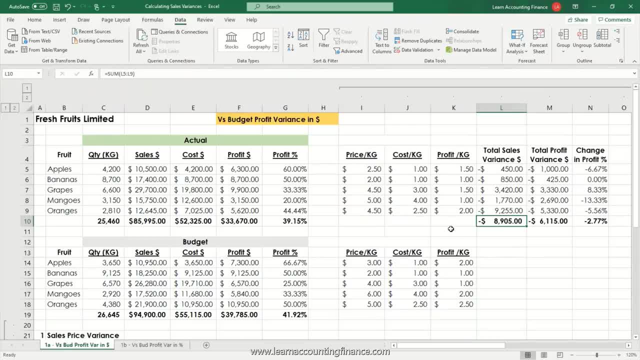 And we will do that, Don't worry about it. Once we set up this file, it will just be a copy and paste and just changing a few inputs, few key inputs, and all the calculations will be done automatically. So don't worry about that. 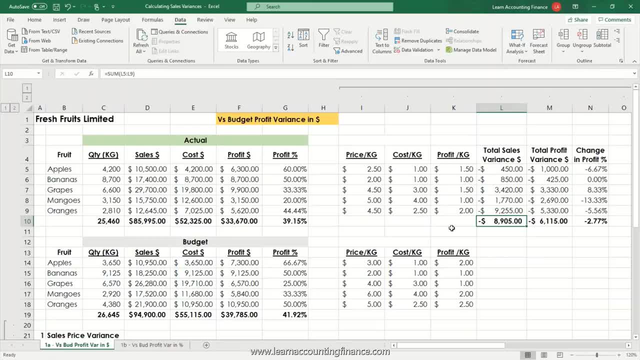 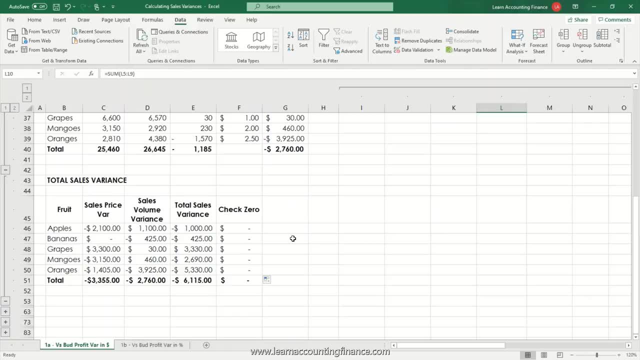 But I think it's really important that you understand this concept And once you understand that it's so easy to calculate those variances, So well, we are done with our first layer of variance calculation. You should be feeling very happy, very excited, that you can easily explain now the total. 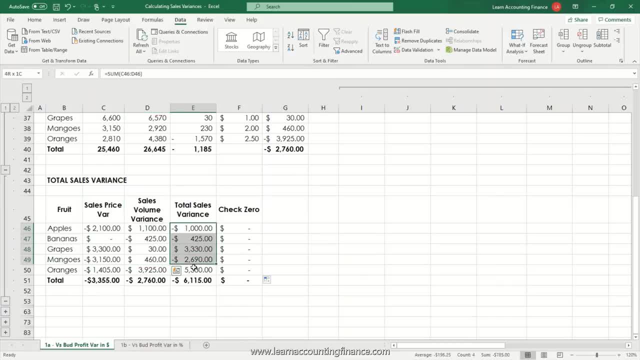 change by price and volume in terms of dollars already. Right, Think about it. If you go back and apply this to your organization, your business, wherever you are, you can tell exactly what's going on as far as the total drop in profit or total gap in profit is coming from. 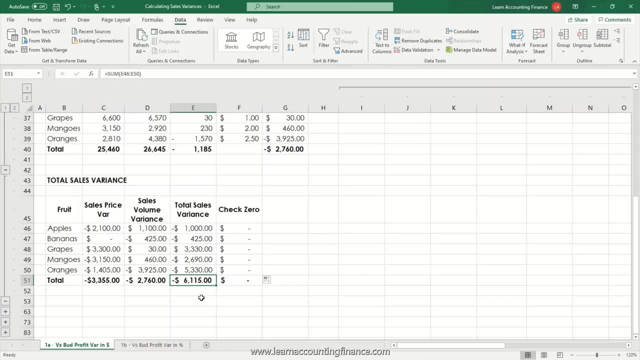 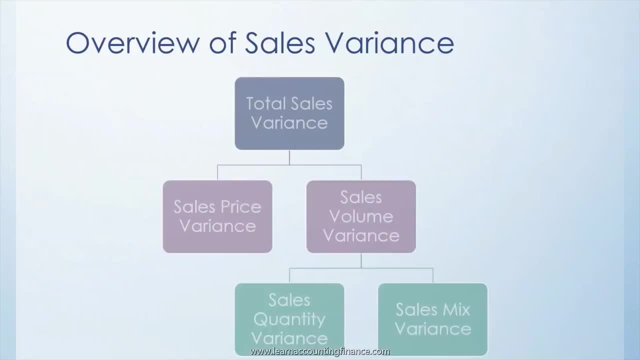 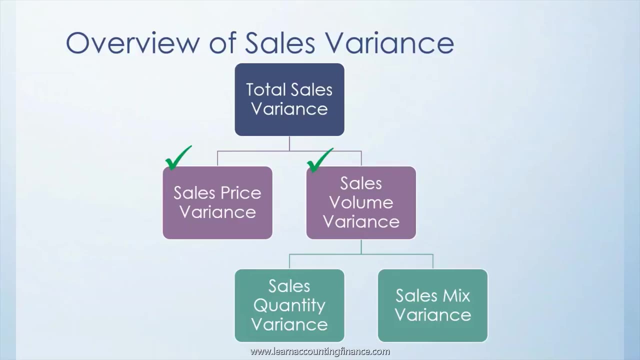 This is great, Exciting. Let's keep going and let's try to explain this even further. All right, So we are making significant progress. Where are we right now? We have calculated sales price variance and sales volume variance, and we have also ensured that the sum of the two 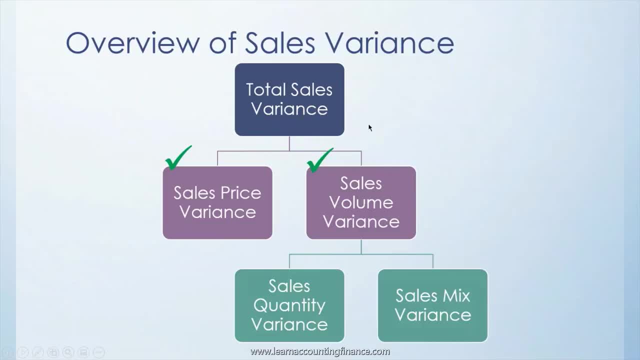 the total of the two agrees to our total sales variance. Now it's time to look at further subdivision of sales volume variance, which is the sales quantity and sales mix variances. Let's focus on sales quantity variance for now. Let's go back to our Excel sheet and 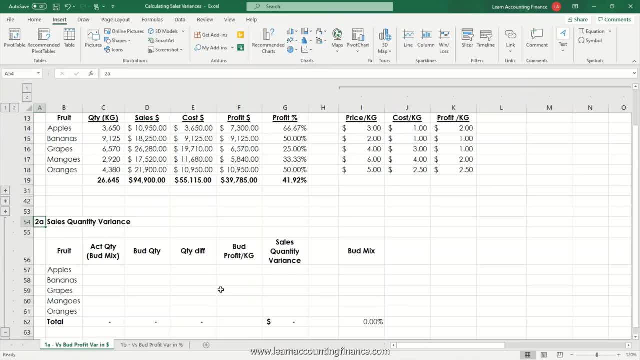 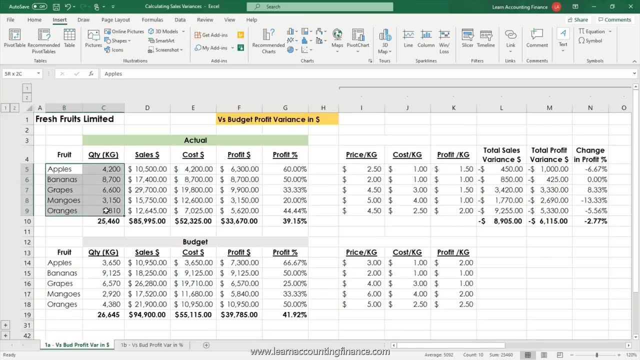 try to calculate sales quantity variance first. At this point it is important to understand the concept of mix. So what is mix? If you look at our actual and budget data, you see we have different products. We have about five different fruits that we sell or that Fresh Fruit Cement sells. 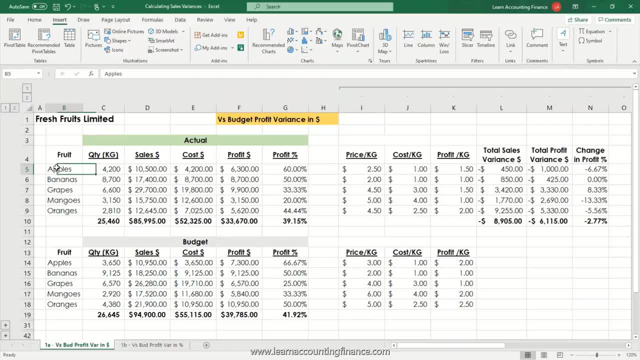 What mix represents is the percentage of each fruit within the total quantity. So, for example, if we sold 4,200 apples out of 25,460, what does that represent in terms of percentage? The same thing for budget. So let's calculate the budgeted mix. 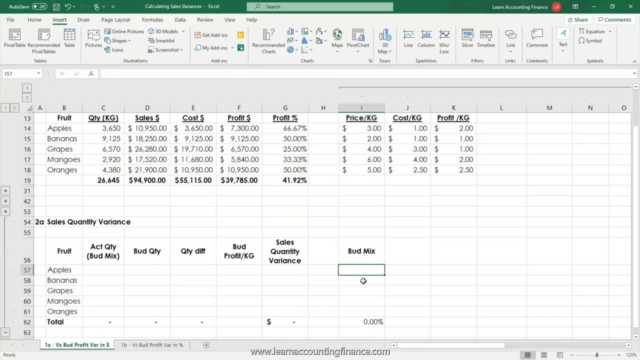 The budget mix. for example, how you will calculate is: take your actual sales for apples and simply divided by the total sales, total budgeted sales, And I'm going to free the cell C19, representing the total sales, so that once I copy the formula down, 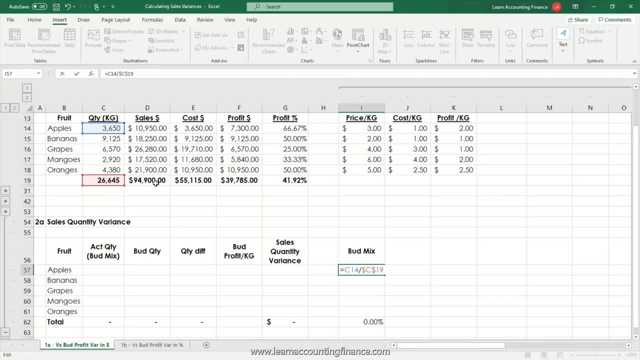 it does not change the cell, it locks the cell. So you can see the percentage of sales for apples is 13.7% And if I copy this down now, you see percentage or mix for all of the different fruits And the total should always be 100%. 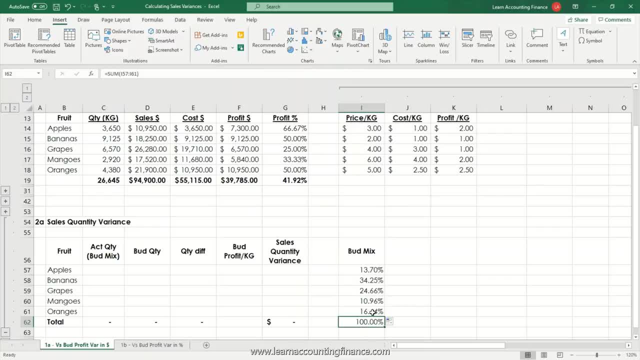 If it's not 100%, then it is wrong. Going back to freezing the cell, as you can see, cell C19 was frozen with putting two dollar signs behind C and 19,. column C and row number 19.. That's why when I copy the cell downward, it doesn't change. 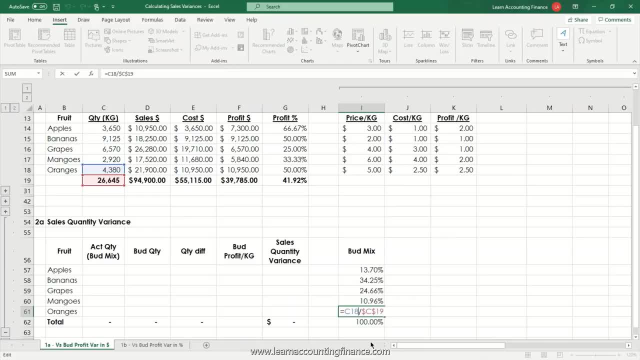 It is always the same. However, the cell that I did not freeze keeps moving as I copy the cell down. Just a little bit of information there if you already did not know that. So anyway, if you have the mix, this is budget mix. 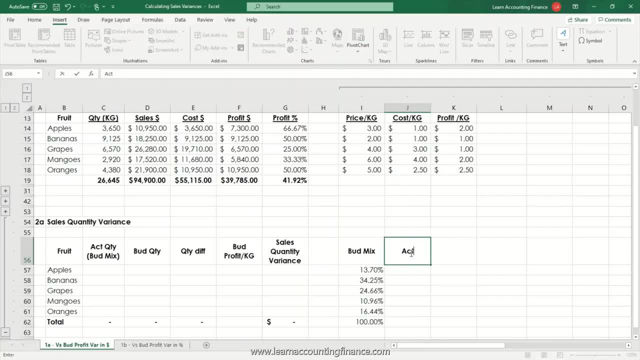 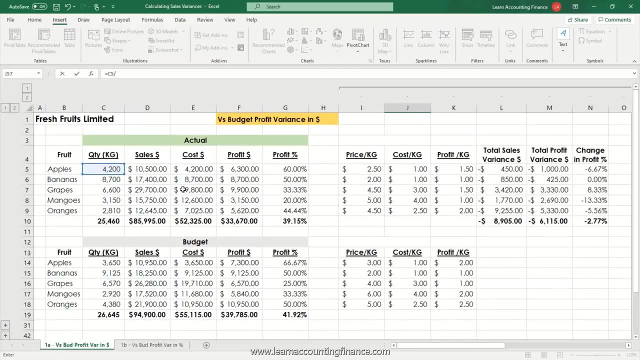 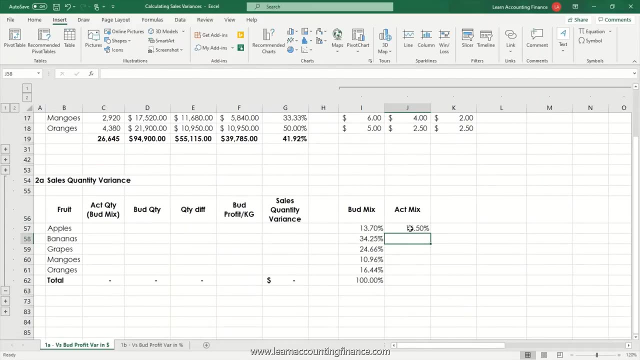 Now, if I have to calculate actual mix, just for reference, I can calculate actual mix in the same way as well. Let's look at our actual quantity divided by total actual quantity And again I'm going to freeze the cell C10 in this case, drag it down. 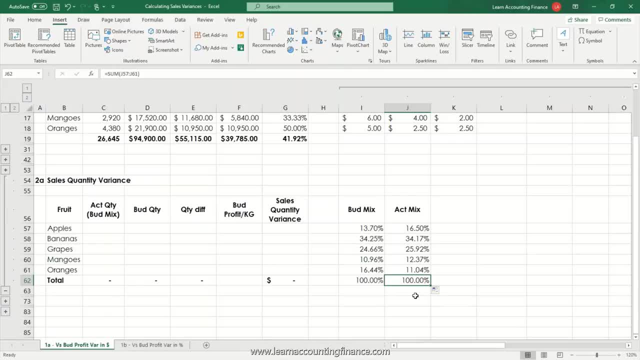 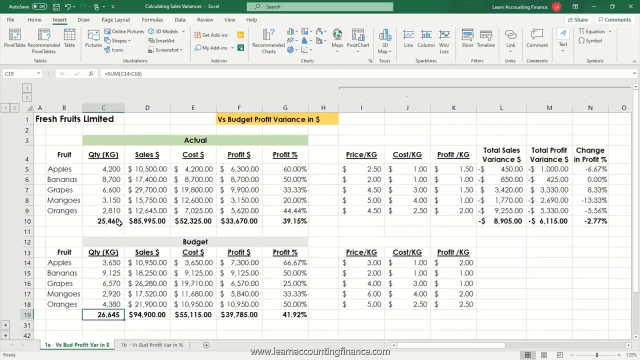 and drag this formula, which is the sum formula. Again, it should be 100%. So you see there is change in mix. Not only is there a change in the total quantity sold. we had budgeted quantity of 26,645 kgs, but we actually sold 25,460. 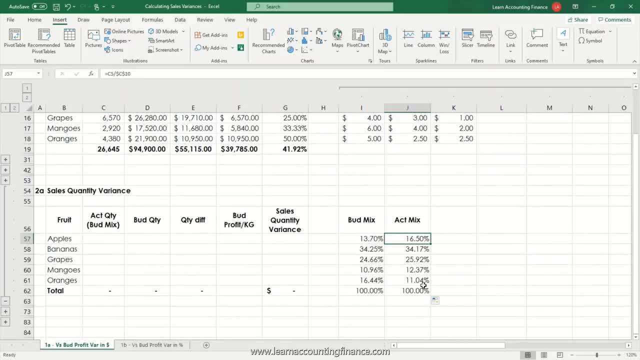 But not only that, there's also a change in the percentage of mix for each fruit. So, for example, in our budget we expected about 30.7% sales related to apples, But actually we did a higher percentage, which is 16.5% in actual. 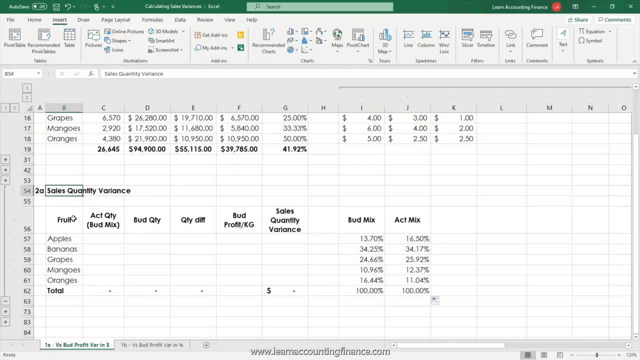 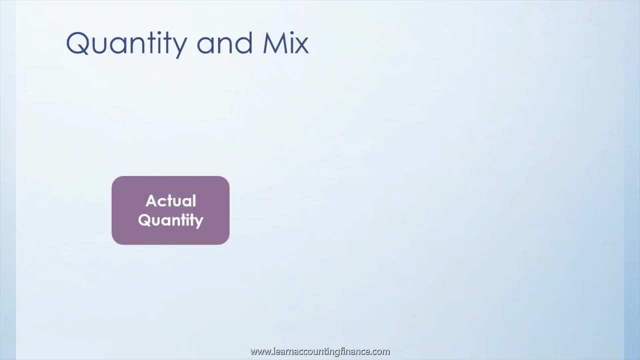 Now, when we are going to calculate quantity and mix, we have to understand this, We have to really. we are really comparing three different measures. What are those three measures? So what we have is actual quantity, We also have budget quantity, And then in between there is a mix which is actual quantity at budget mix. 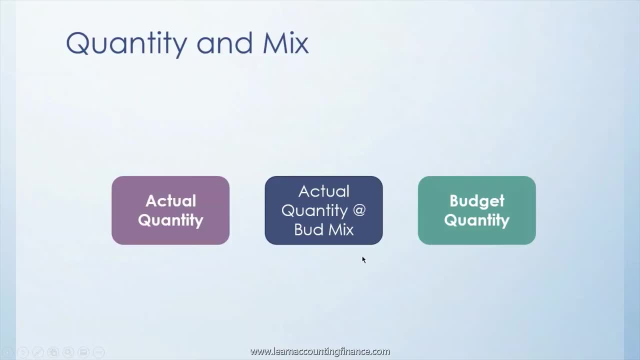 And then we have the actual quantity at budget mix. So again, if you have a budget quantity or a budget mix, you should remember these three boxes when calculating the volume variance and quantity and mix variance. So again, we have actual quantity, we have budgeted quantity. 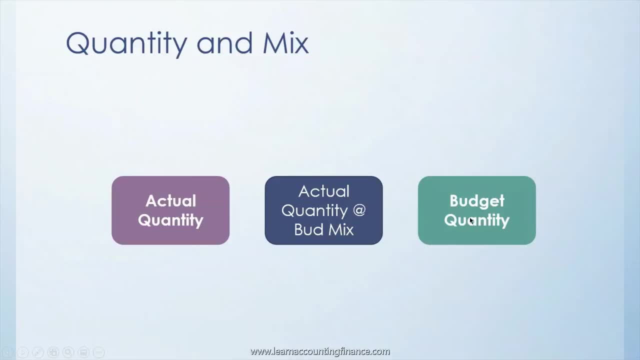 and then we have a mix, which is actual quantity at budget mix, And then the difference between these two, which is budget quantity and actual quantity- difference between actual quantity and actual quantity at budget mix- gives us our mix variance. and then together, all of these variances combined give us our 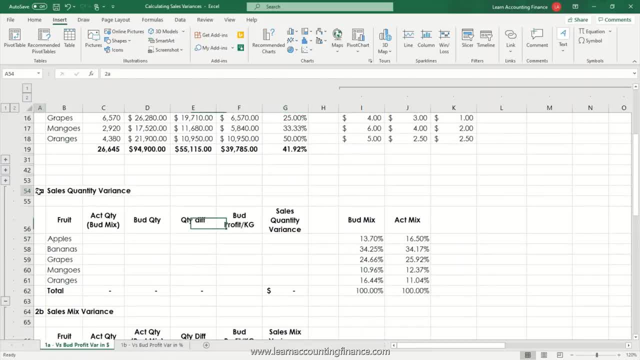 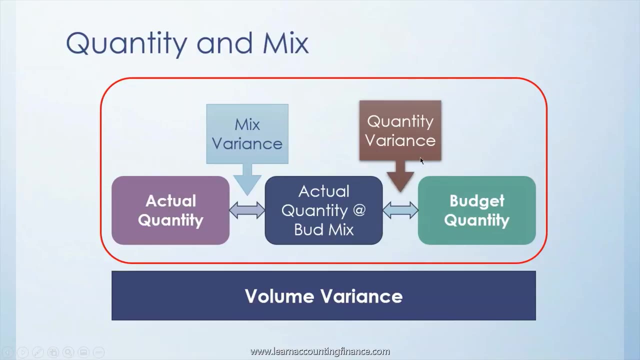 volume variance. so, going back to our example, we are at the point where we want to record the sales, we want to calculate sales quantity variance, as you can see, which should be the difference between budget quantity and actual quantity at budget mix. as we're calculating quantity variance, we know 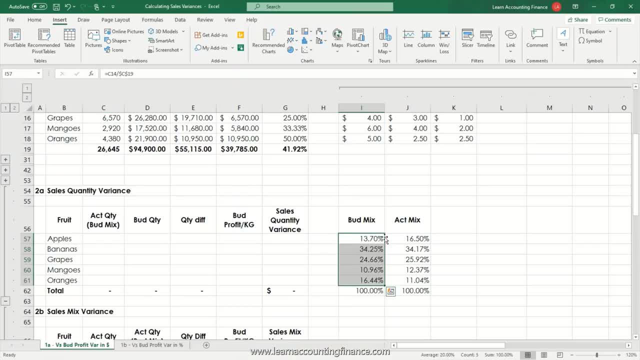 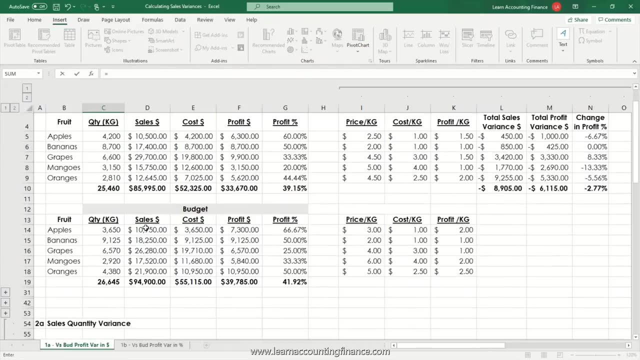 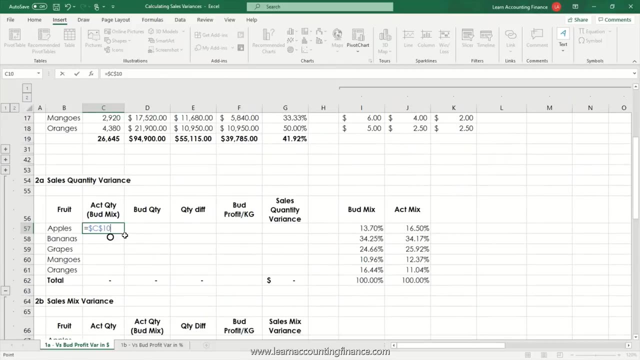 we just calculated budget mix here in this column, so how we will calculate actual quantity at budget mix. this will be your total actual quantity, which is twenty five thousand four hundred and sixty, and once again I'm going to freeze the cell times: your budget mix gain. what is it your actual quantity, but at budget? 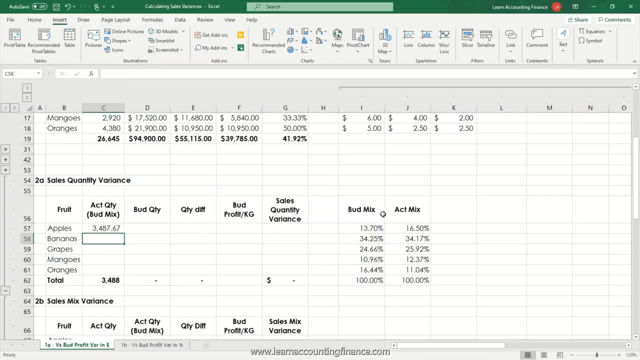 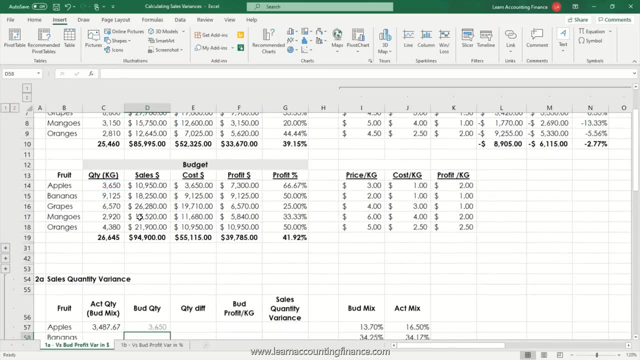 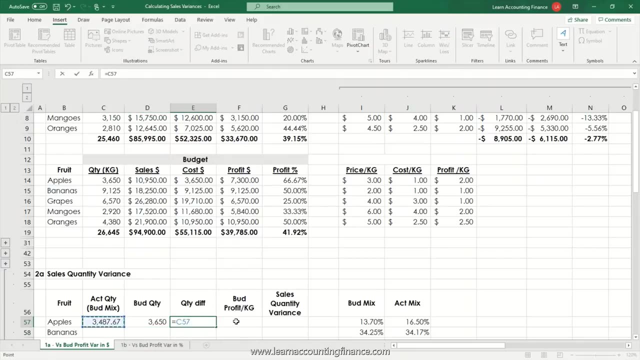 mix, not actual mix, right? and then budget quantity is simply your budget quantity, so you will simply link it to your budget quantity and then again you have a quantity difference which will be actual quantity at budget mix, minus your budget quantity. here you will use profit per kg, budgeted profit per kg, again, in fact, in calculation of 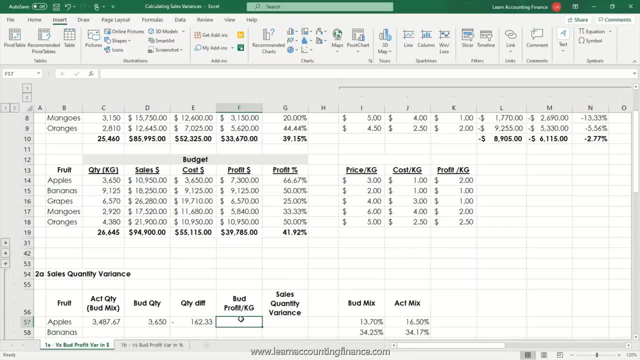 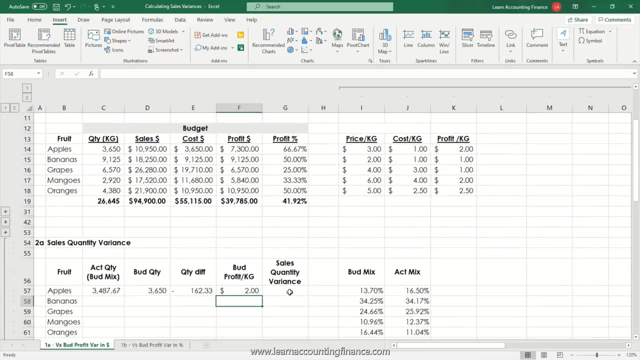 all three: volume, quantity and mix. you will always use the budgeted profit per kg if you are comparing variances against budget. so let's link it again. we know the budget profit is in this cell and we have now our sales quantity variance which will be budgeted. 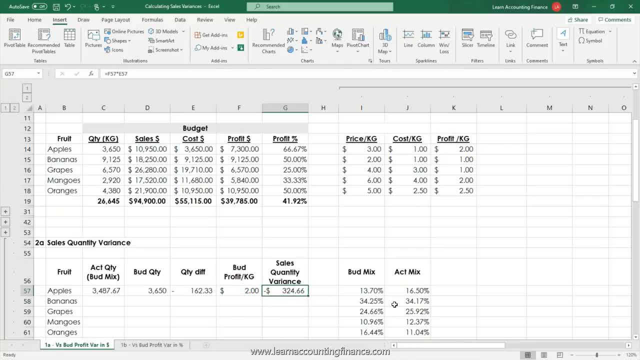 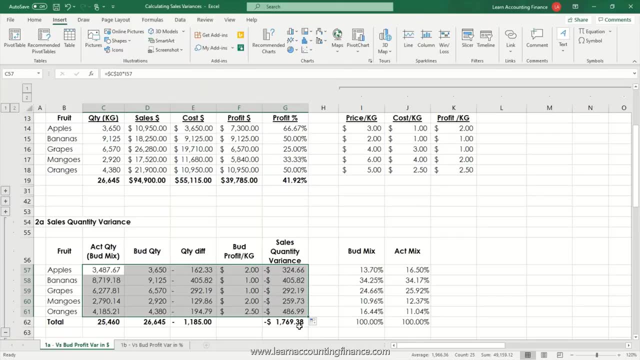 profit times the quantity difference, and we can drag all of this down to calculate variances for each product and this gives us our total sales quantity variance of 1769, and there are some 38 cents as well, because now mix is being involved and Excel is doing the calculation for us. 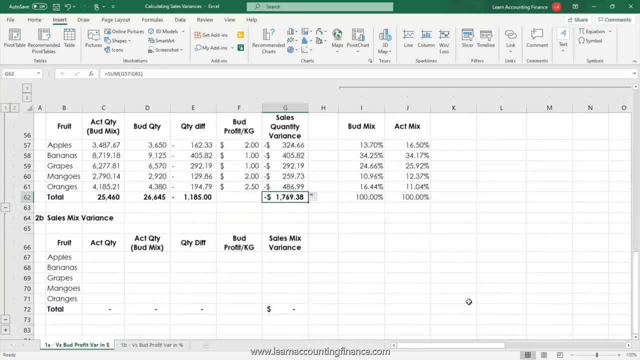 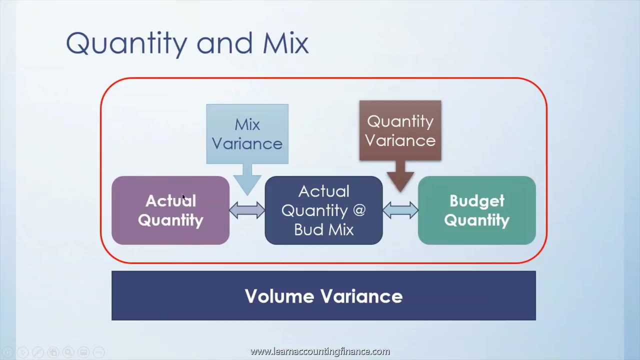 let's do sales mix variance as well. so what did we say? how is? how is sales mix variance calculated? let's go back to our slide again. so mix variance is the difference between your actual quantity. by the way, you can also calculate your actual quantity. by the way, you can also call actual quantity as actual quantity. 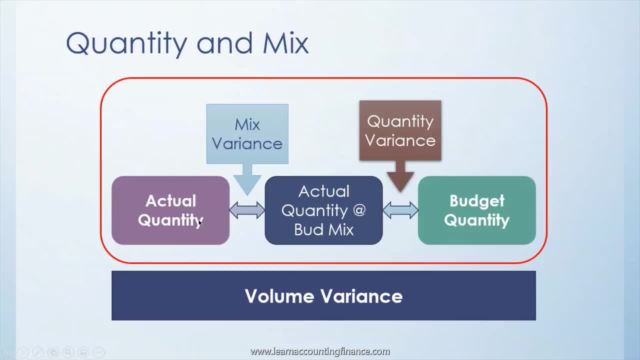 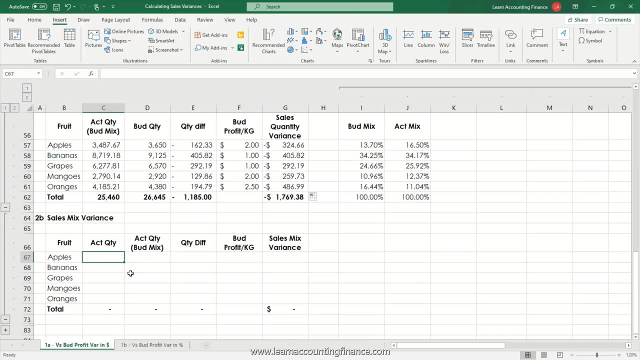 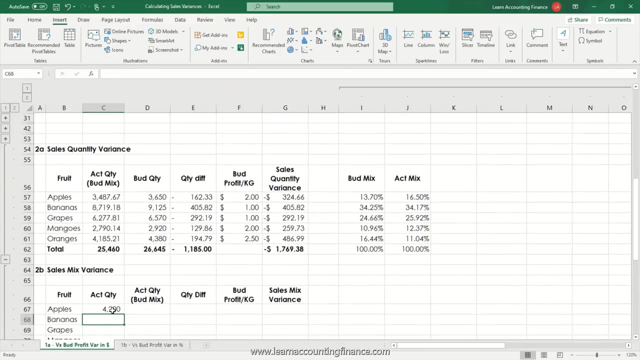 at actual mix. right, it's the same thing, but it will be the difference between your actual quantity and your actual quantity at budget mix. this will give you your mix variance. so we have actual quantity already in the data. let's link it to the actual quantity. we have actual quantity at budget mix, which is already. 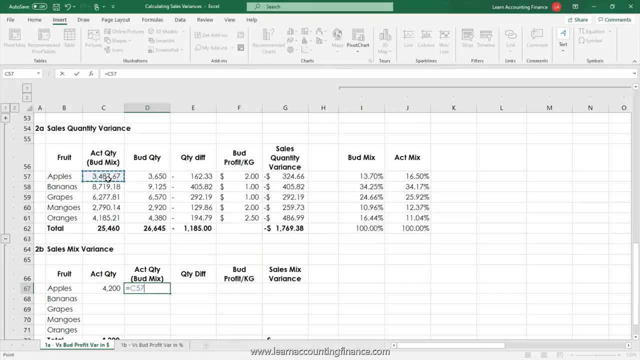 calculated here up here. you can simply link it to the sales above and we can calculate over quantity difference here as well, which will be your actual quantity minus your actual quantity at budget mix. going back to budgeted profit per kg. you can take this number as well, you can refer it to. 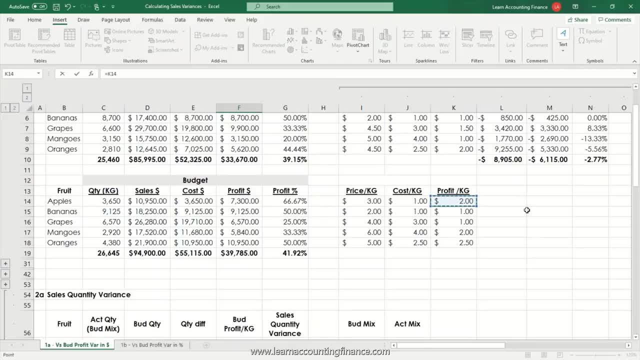 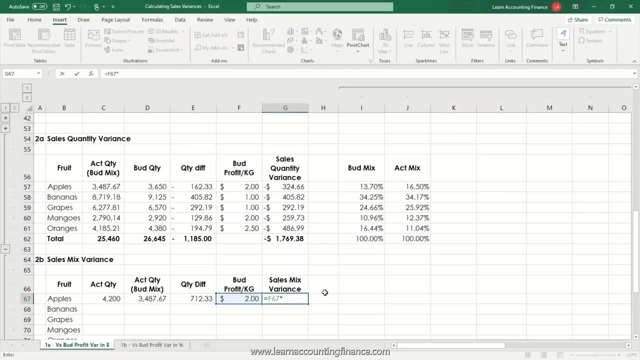 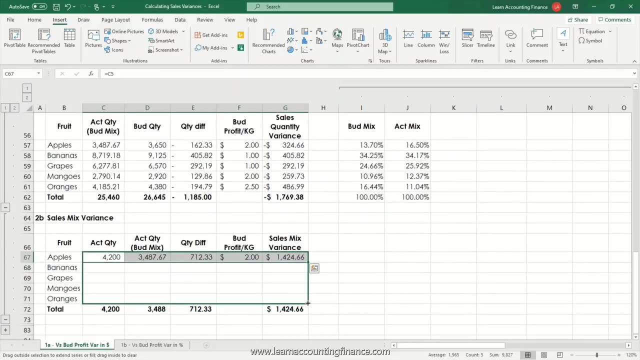 this cell or you could go up and refer it to the budget profit per kg calculated above, and then your sales mix means: is your budgeted profit times the quantity difference and this gives you your sales mix variance. now, if you scroll down, if you copy the cells down, 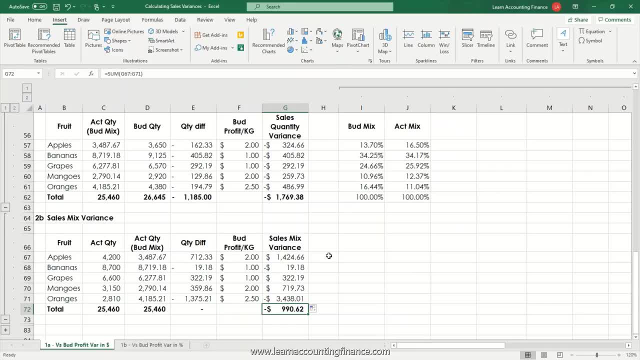 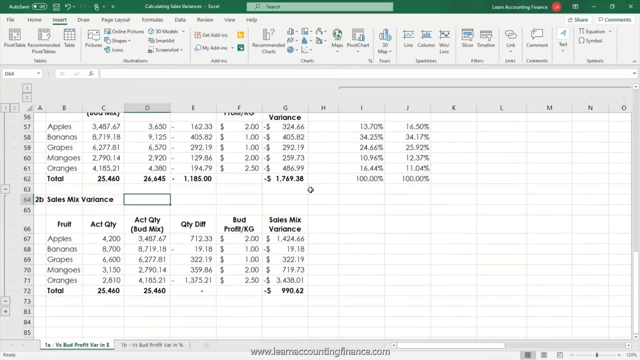 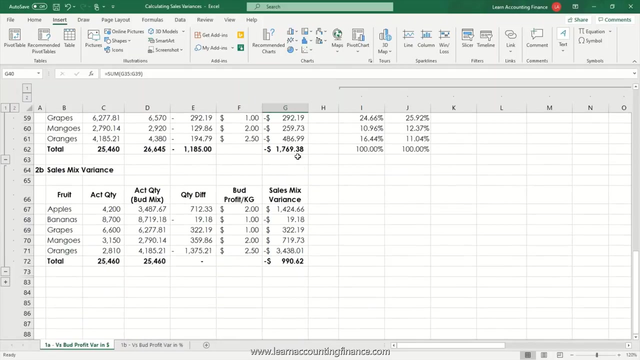 you will get your total sales mixed variance. at this point you want to do another check. as you know, sales volume variance is the sum of sales quantity variance and sales mixed variance. let's do a quick check here again. we know our sales volume variance was $2,760, right, and if you add this sales quantity and sales mix and you have here again $2,760. 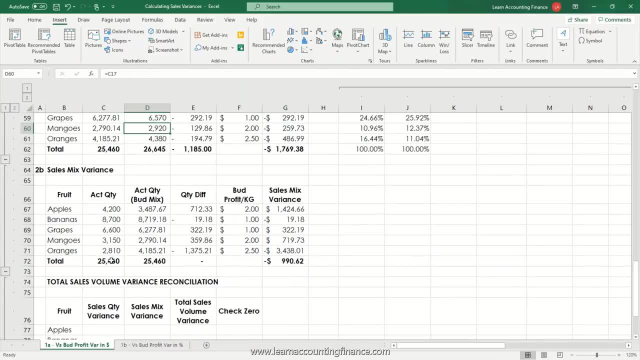 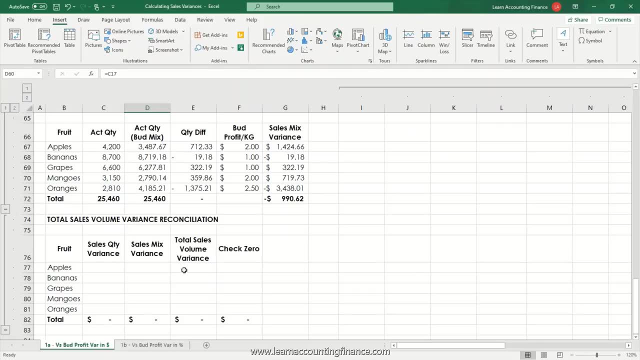 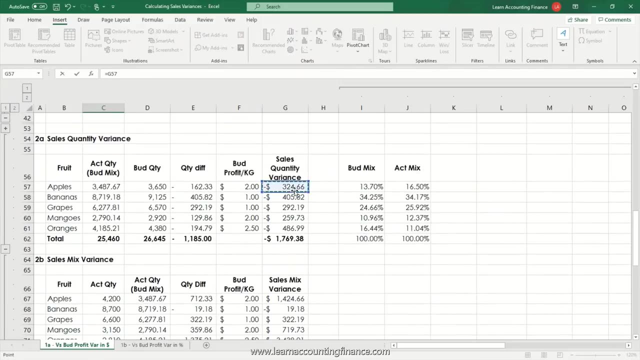 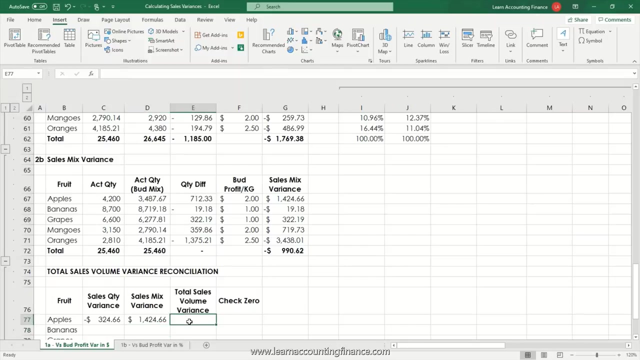 so again, it works, it matches. it's time to do a total volume variance reconciliation. we do it um in a similar fashion as to the reconciliation we did earlier. so, as far as sales quantity is concerned, we have apples um sales mix and then we have total variance, which is the sum of the two, and then we can. 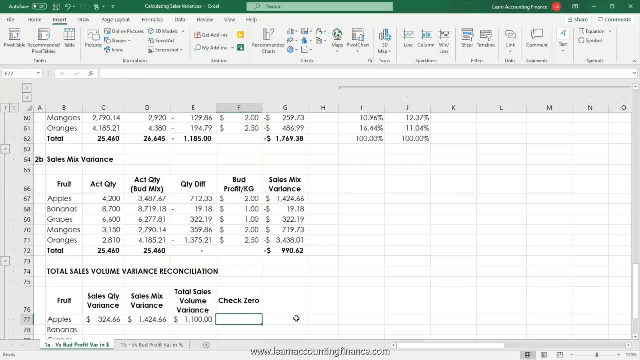 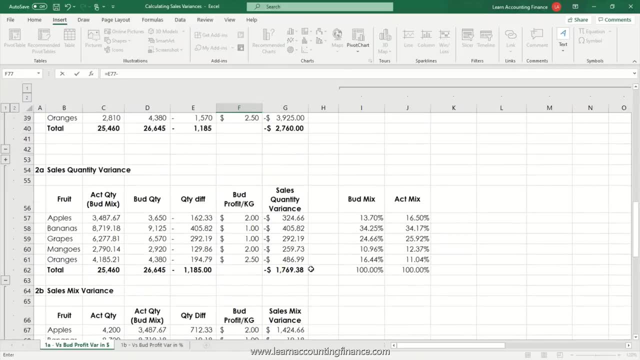 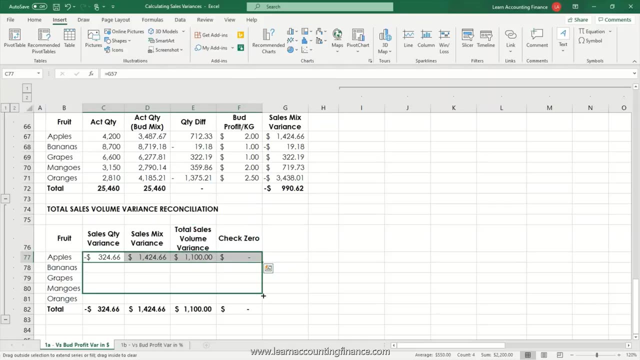 again check this: uh, volume variance. so this will be the volume variance as a sum of two minus the volume that is calculated. here again, the check shows a zero. from my experience, it's always good to put checks and balances, because sometimes we make mistakes unknowingly, unintentionally, and then we are so deep in our analysis that it comes and bites us. 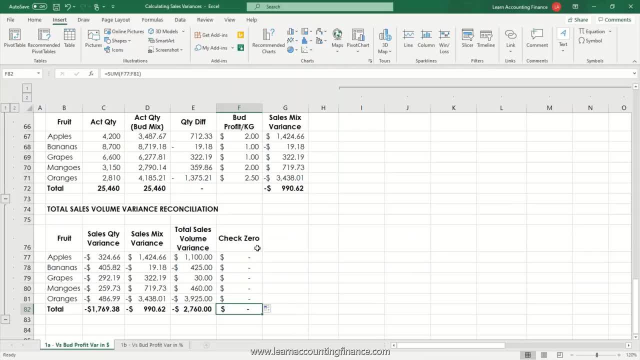 back later. so my advice to you at every step: it's very quick, you can quickly put those checks in place, and the checks should always be done in a way so that you you can see a zero in there and you can be sure that the calculation is done perfectly. 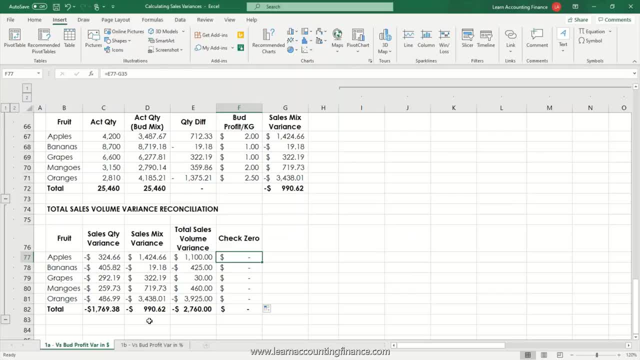 anyway. so our volume reconciliation is also done and, as we can see, we have by foot or by product the variances in place and we see that they match in total. we already did a total reconciliation of sales price variance and sales volume variance, which matched as well. so in our way, if we go back to our overview, we have now calculated all. 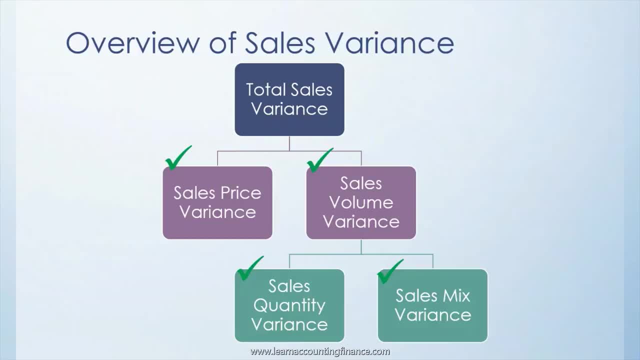 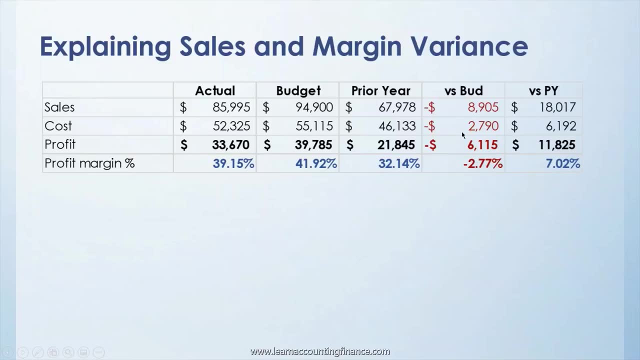 of the variances. um, you have calculated sales price and sales volume and we have seen the spread between and sales mix. so we are done explaining the six thousand one hundred and fifteen dollars right? so overall we can clearly explain the change versus budget or the gap versus budget as far as profit dollars are concerned. but we haven't. 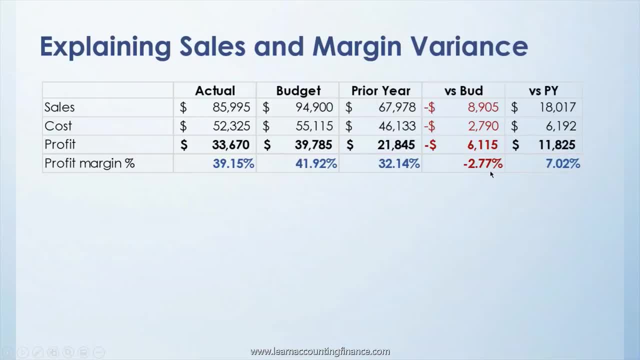 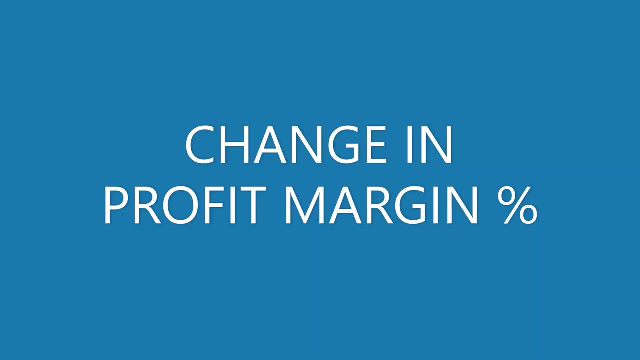 explained the drop in profit margin of two point seven, seven percent. yet in the next few sessions we are going to discuss and calculate exactly that. we'll see how this is calculated and what is the result. welcome back. so at this point we have already explained the change in profit. 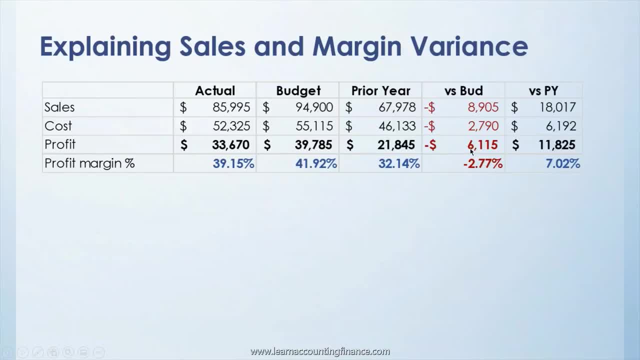 dollars as a result of sales variances. now we are going to look at the change in profit margin, profit percentage. what is profit percentage? it's really your total profit divided by your sales. so in this case, when you see thirty nine point one hundred and fifteen dollars, you will see that the profit margin is. 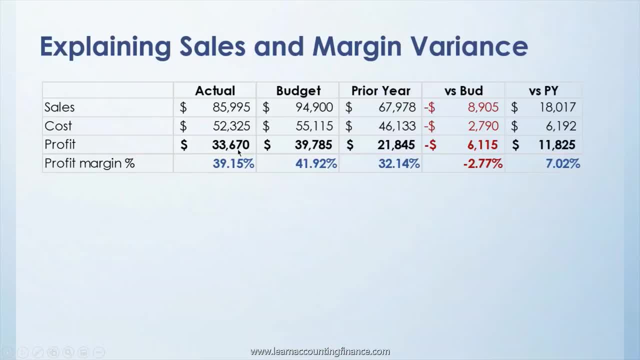 one five percent. this is really thirty three thousand six hundred seventy, your profit divided by your sales of eighty five thousand nine hundred and ninety five, and the same for budget and prior year. again, we are still in the budget scenario, we are still explaining versus budget. but the good thing is as we are. 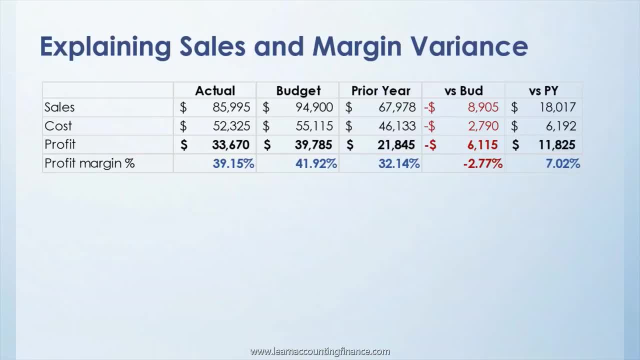 building these files. we are building this excel file. we are greatly reducing the amount of time we will need to spend later, when we start calculating the same for prior year, and you will see how quick this will be. well, my friend, i hope that information that you have seen so far you. 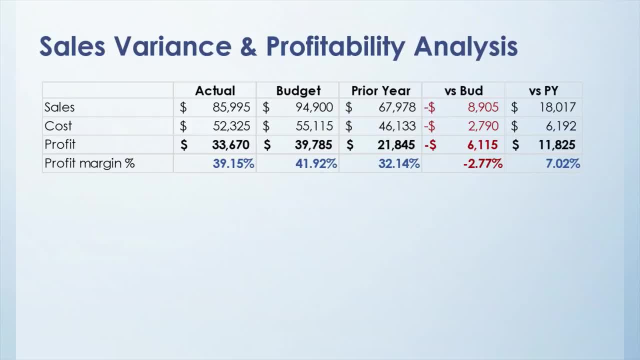 found it- you spoke, beneficial. we still have a lot to learn. so far we have explained to achitations in profit versus budget, but we still need to go along. we need to explain the biggest in profit percentage versus budget, to explain the winnings in sales dollars and sales its cost. not only that, we have